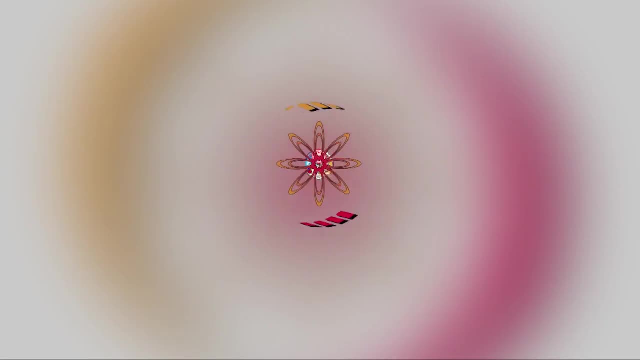 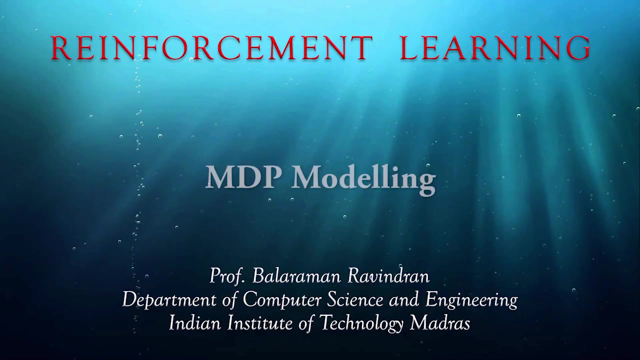 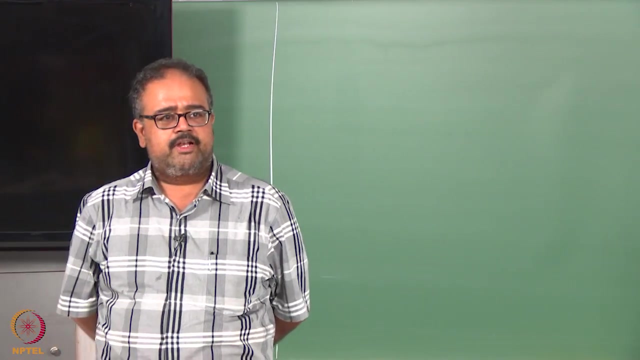 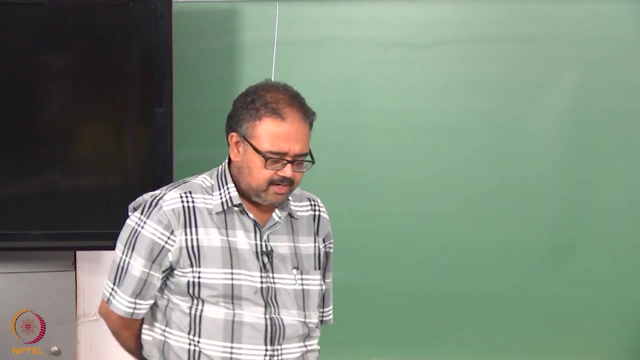 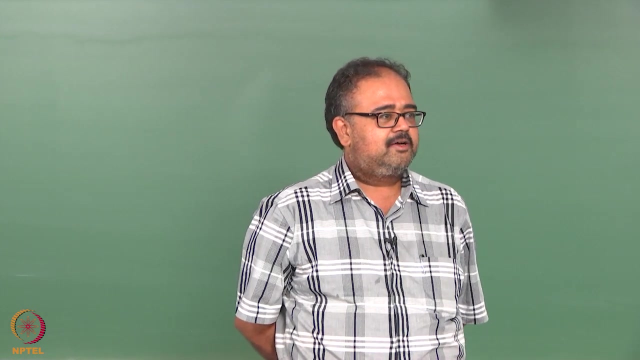 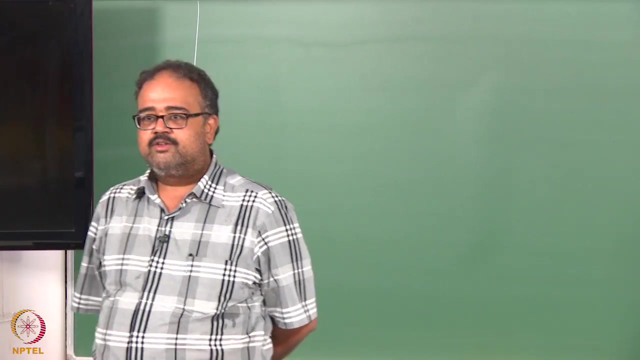 So we will continue looking at the reinforcement, the full reinforcement learning problem. So we left off where we defined a Markov addition process right, and so today's class will probably be a short one. okay, because the next thing, next topic I need to start requires me to define a lot of notations and stuff like that. So if I start that today, I will 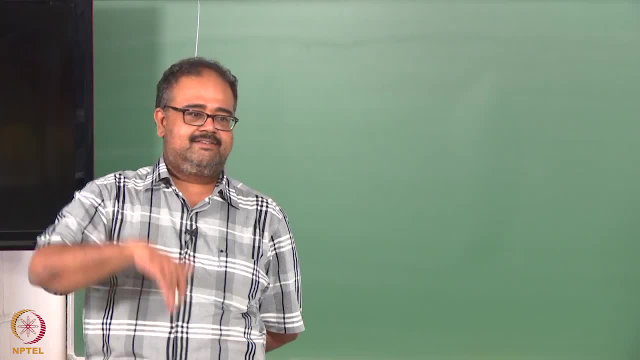 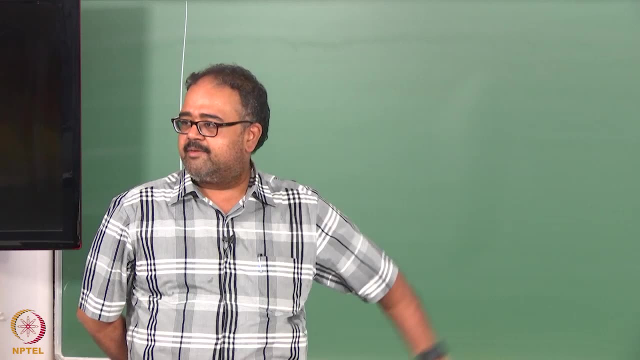 probably end up just defining the notation today and then when I start again next week I will ask you. I will have to ask you to recall the notation and stuff like that or spend time writing it out again. So I will not do it. so if I finish whatever I want to before, 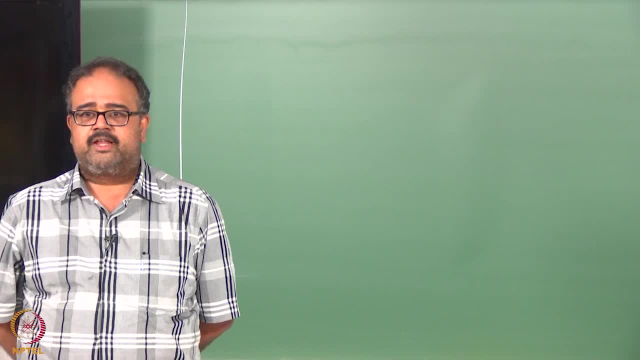 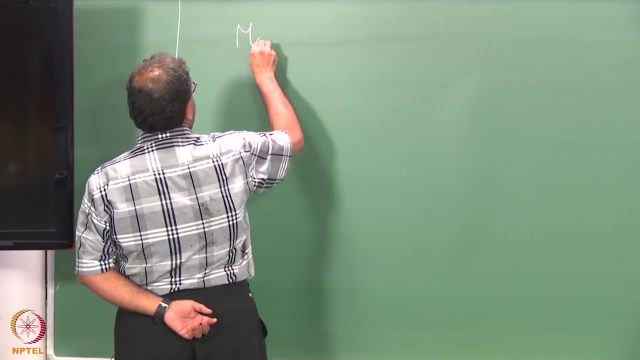 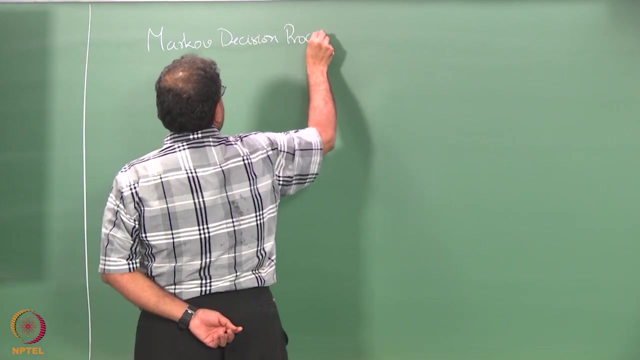 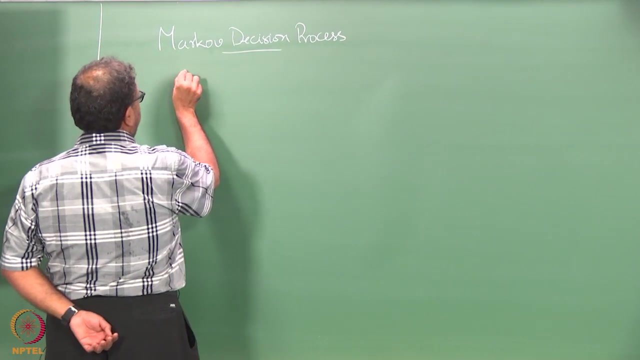 the proofs start. right. I will just stop today so I will not start the notations. okay, So let us see how it goes. So so we started looking at the Markov addition process last time, so we said that it is specified by set of states actions. 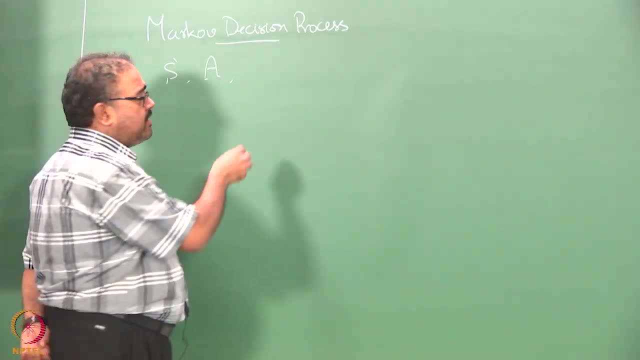 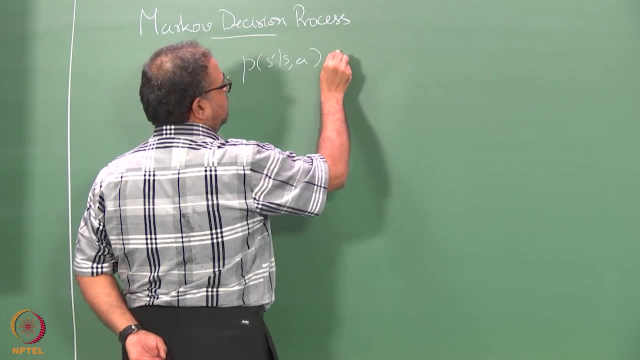 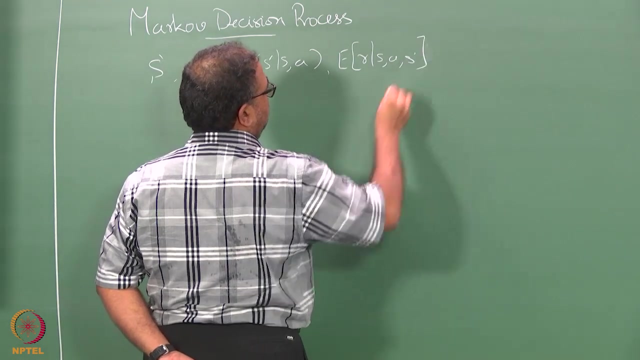 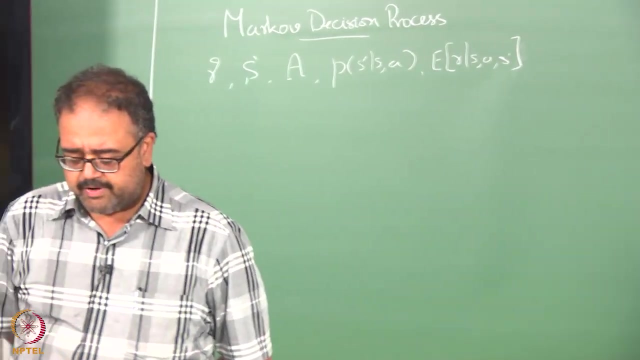 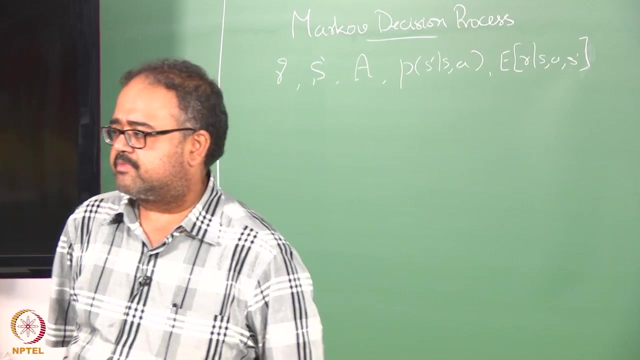 Okay, Okay. So we have two things right: transition probabilities and and possibly a gamma. So if you look at the RL textbook right, they leave out the gamma Okay. So if you look at the RL textbook right, they leave out the gamma Okay. 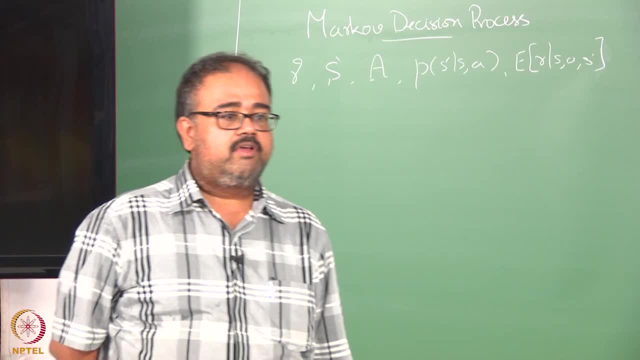 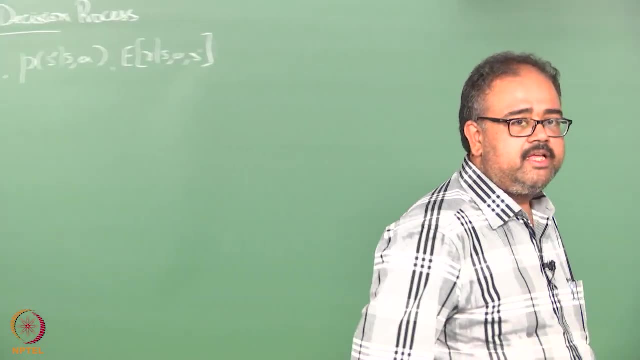 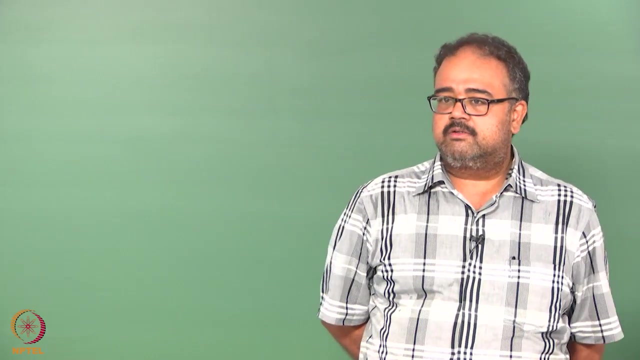 So if you look at any OR textbook where also MDPs are used widely, right, they would have the gamma in there, right. so for them gamma is a very inherent part of the problem. but in the, in the RL books, you would see that they would leave out the gamma, even though. 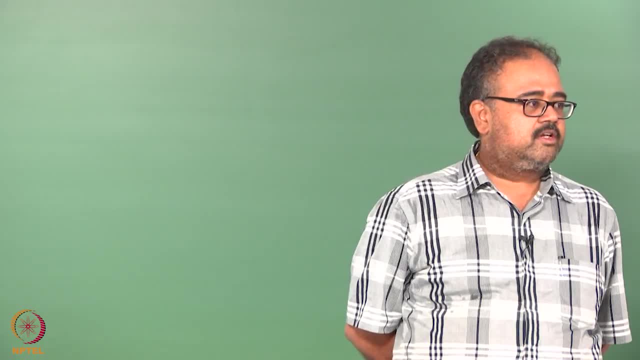 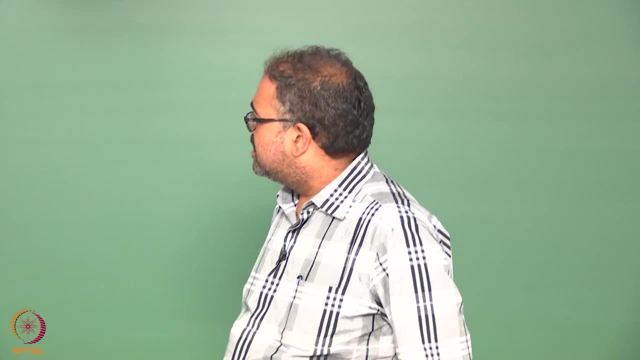 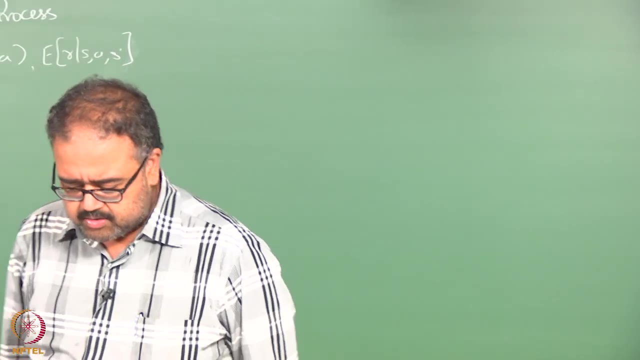 I mean, gamma is an inherent part of the problem. it somehow they just do not acknowledge the fact that gamma changes the solution right explicitly in the problem definition itself. Okay, So let us see what an MDP is all about. So what I will do is walk through one of the examples from the textbook right. 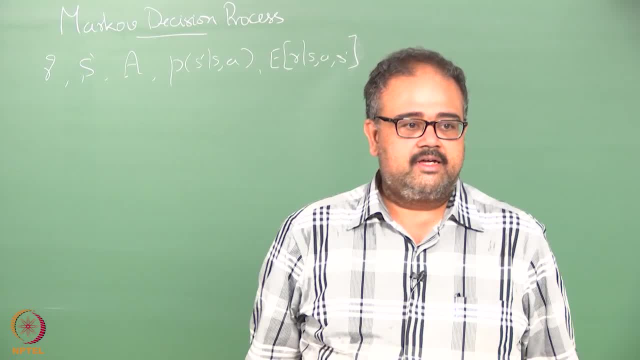 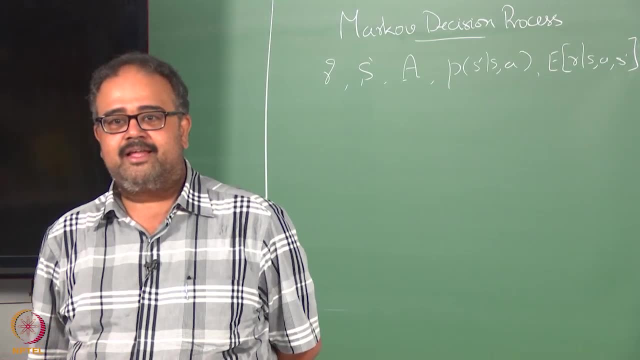 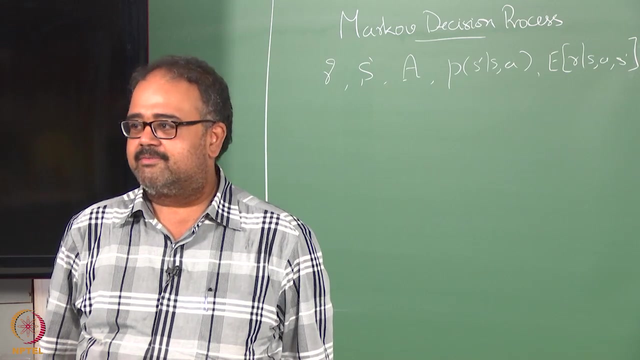 So I mean sticking to the textbook example so that you can go back and read the book and also because it is kind of makes the course more related to the, the minor guys here. Okay, So let us take the example of a recycling robot from the book. 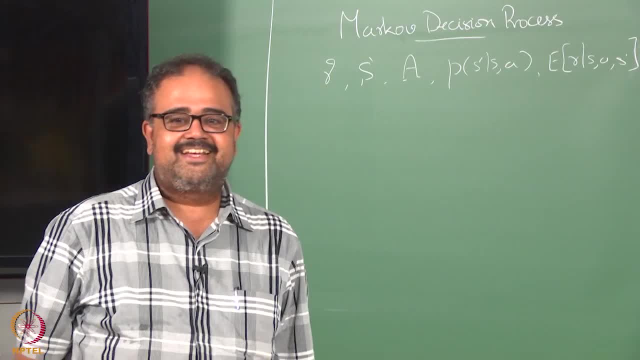 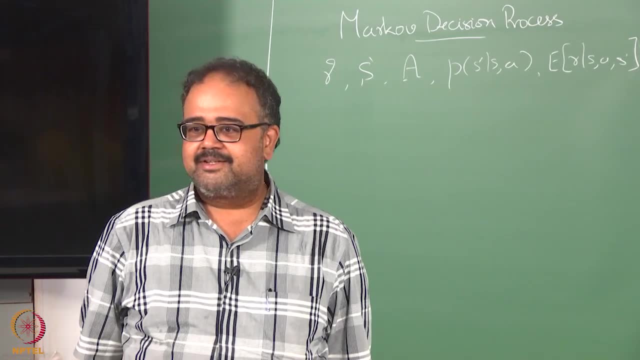 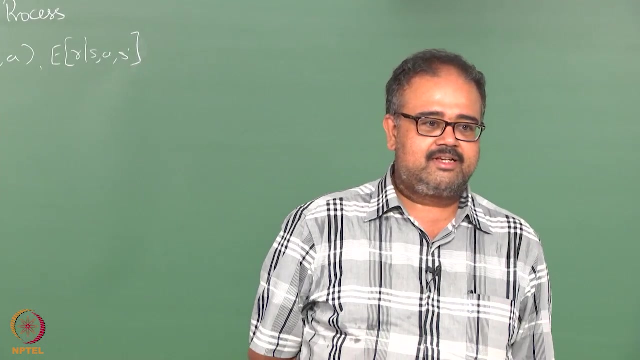 So how many of you have been reading the book? okay, the number went up by two since last time. okay, good, so do you remember the recycling robot? yeah, so what was the thing about? There are three states where it goes and searches for the gamma goes and actively searches for 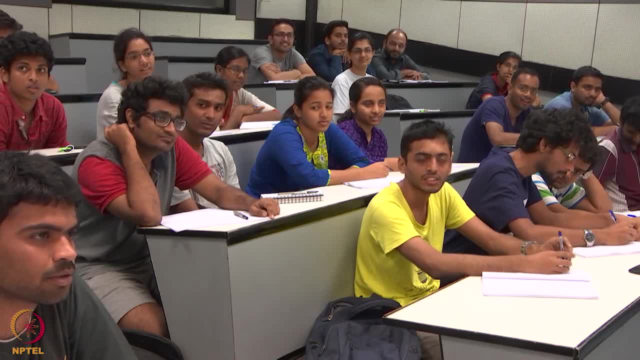 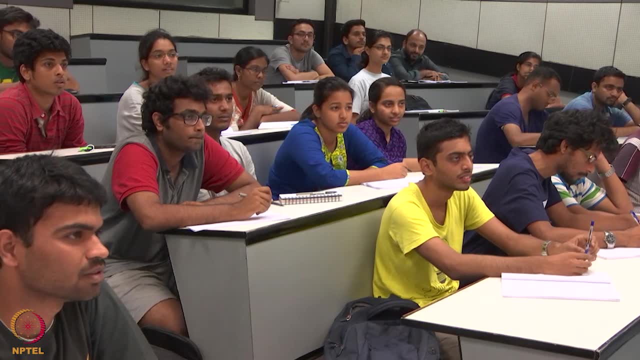 the gamma. the second state is where it waits for some someone to come and leave the gamma, okay, Okay. So it has to take an action between these three states based on the battery level it has and based on that, there will be rewards for that whenever it gets a can, a reward of 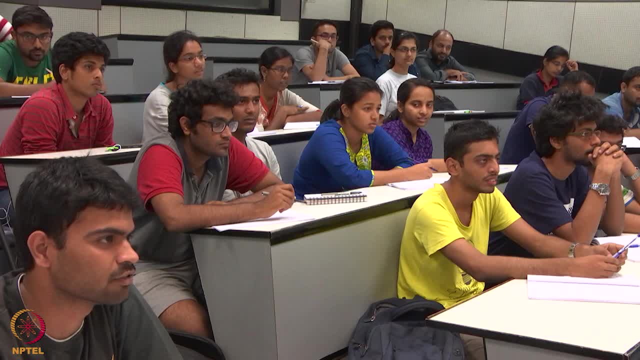 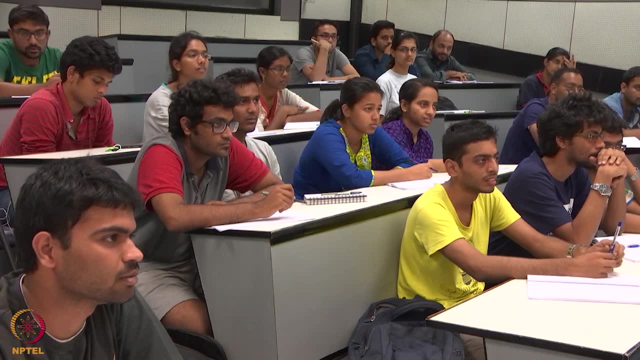 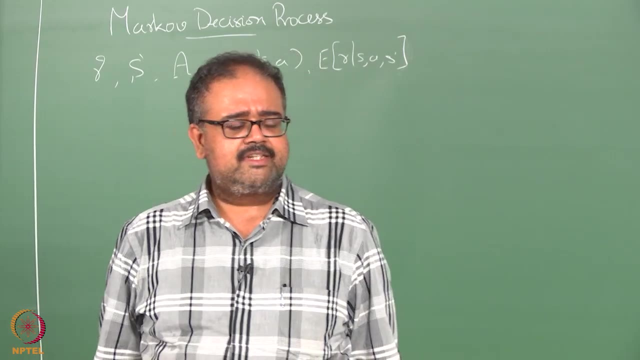 one will be given. Okay. Whenever it runs out of battery, a reward of minus three will be given, otherwise it has to Okay. So it is interesting. Did they just turn on the mic or something you know? it is interesting that you used the description states. 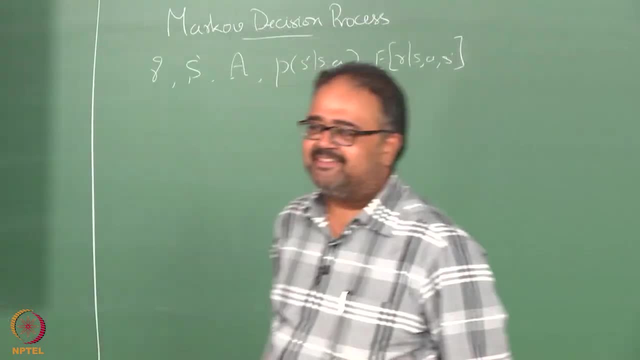 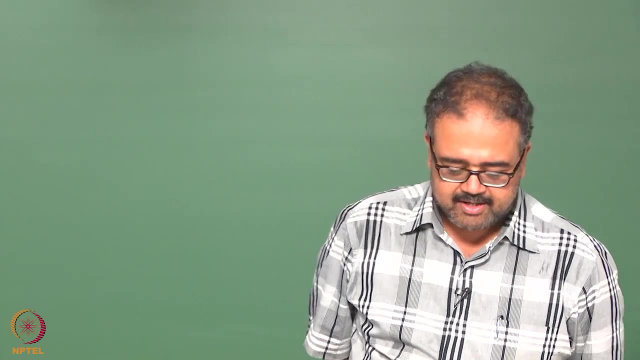 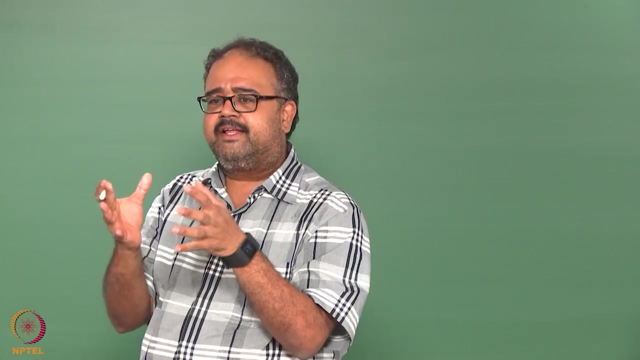 Okay, So people heard him and so I will repeat it, since I seem to have the louder mic. so you know that those can also pick up, but I seem to have the louder mic, so let me repeat it. So that is this robot. okay, that has been created for the express purpose of switch Bharat. okay, 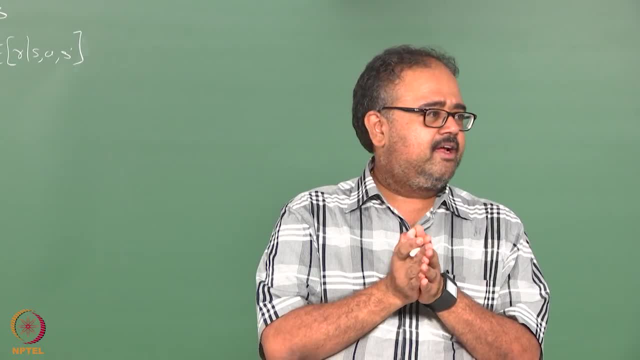 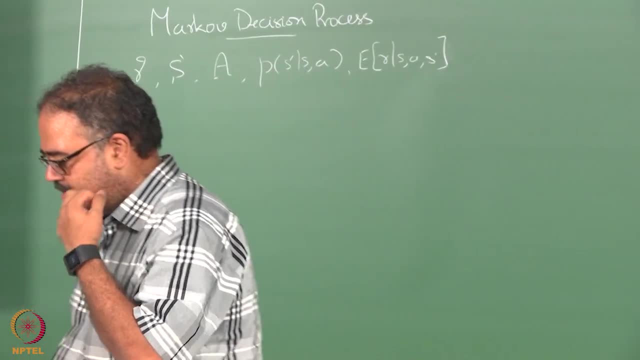 So it goes around the building and finds all the empty cans and gathers it and puts it in some kind of a- Okay, You know, trash recovery system, right recycling system or whatever. So for every can the bot gathers is going to get a reward of one right. this is a number. 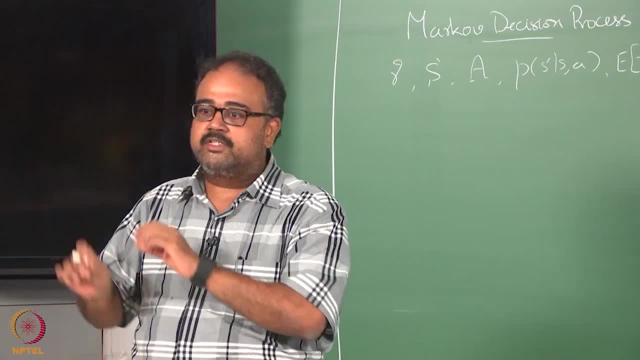 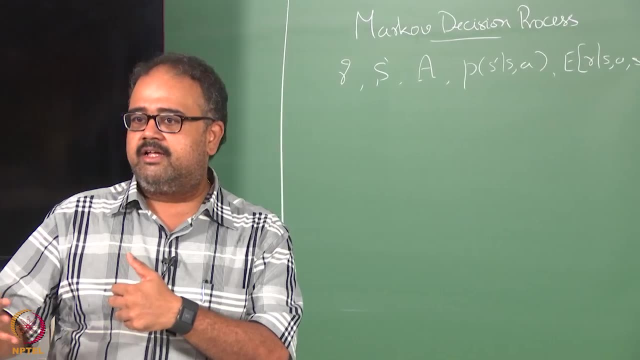 I am pulling out of the hat, right, So let us not talk about the reward now. right, so the robot is supposed to gather cans. that is essentially what we wanted to do, but, being a robot, it is going to have a limited amount of power that it can spend, right? 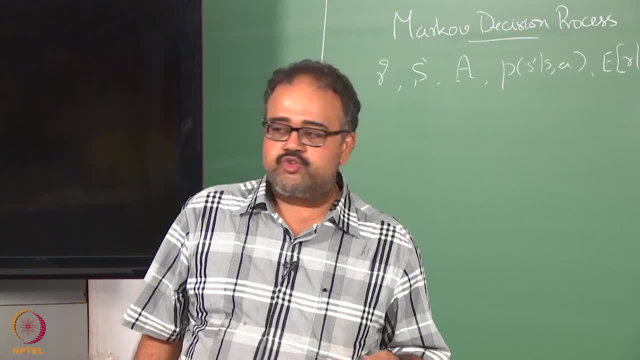 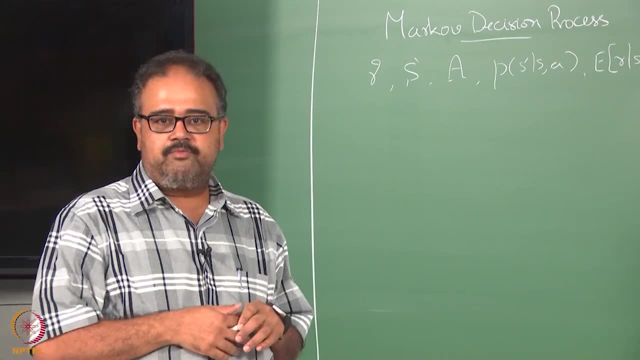 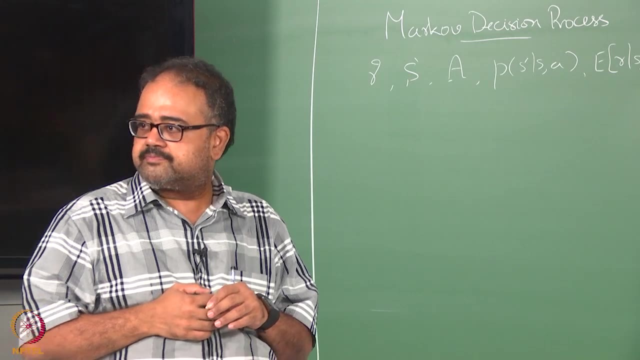 It has a limited amount of battery power that it can spend, so it has to choose carefully how it spends the battery. Right, it can go around looking for cans, right, and if it is going to run out of battery, then it can do one of two things: it can recharge itself right, or it can just sit in a place. 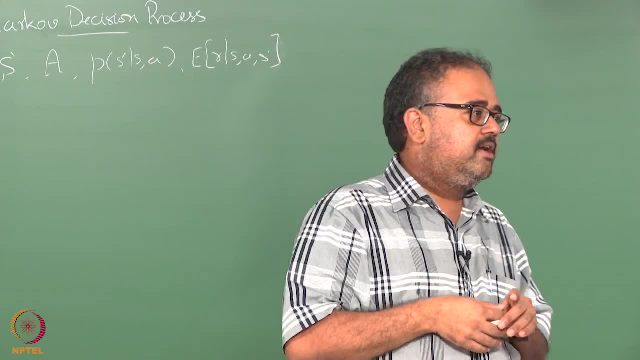 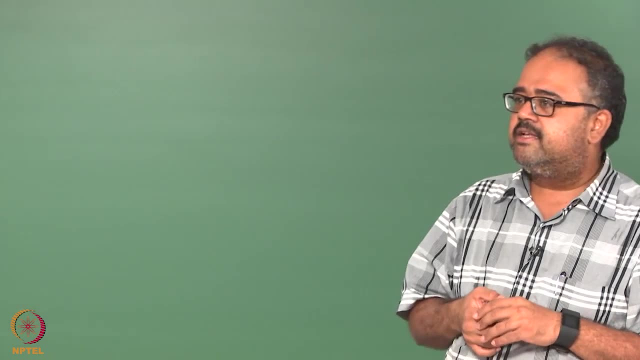 like a trash can and expect people to drop the empty cans into that bot. okay, just sits in a place and people can just use it like a trash can, right? So this is essentially the robot. Okay, Okay, Okay, Okay, Okay, Okay. 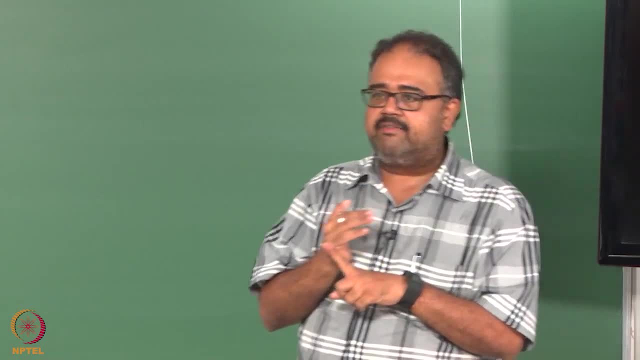 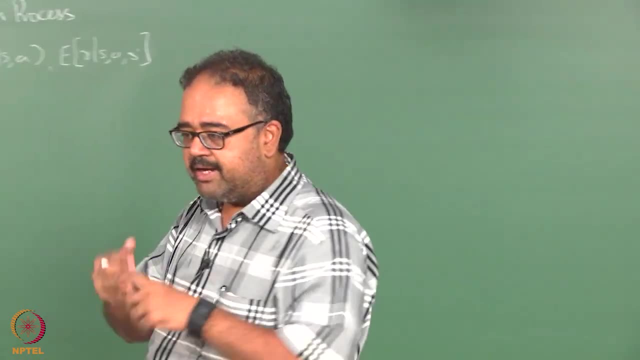 So this is essentially the setup. so I have this bot that should. I would like it to go actively gather cans, but I also do not like it to run out of battery, because if it runs out of battery somebody has to go physically either roll the robot or carry the lift the. 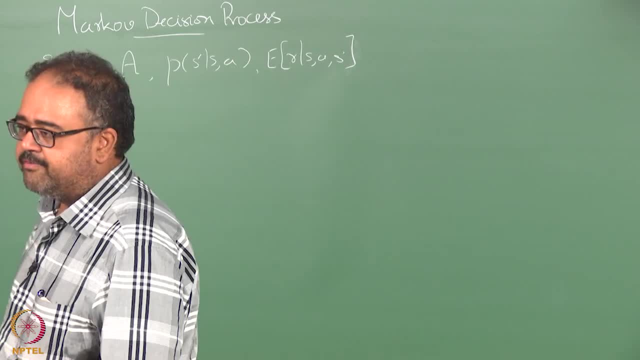 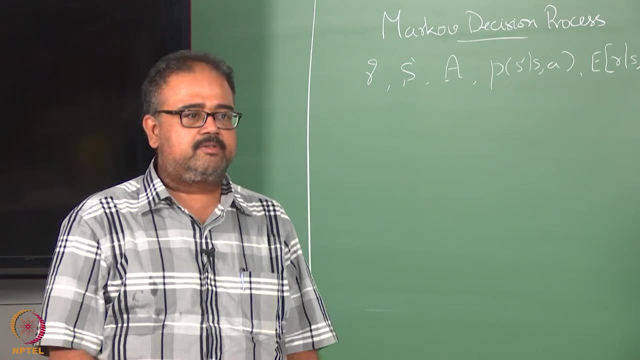 robot and take it to a charging station and charge it. okay, that is a very painful operation, so I really do not want it to run out of battery, but then I do not want it to just sit idle as well, because what it is supposed to do is gather cans, right? 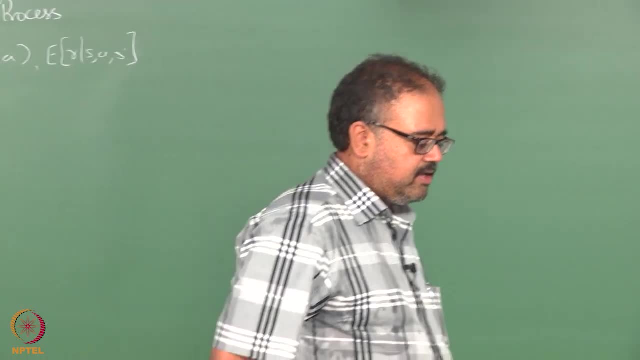 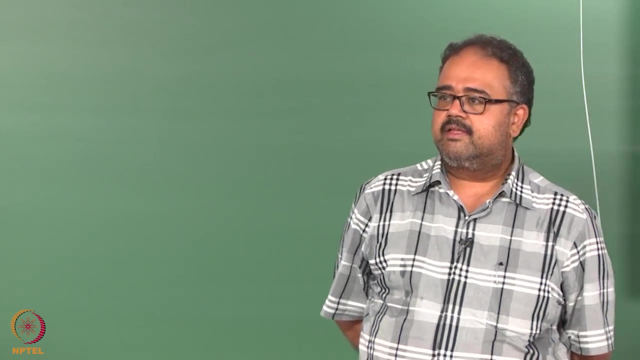 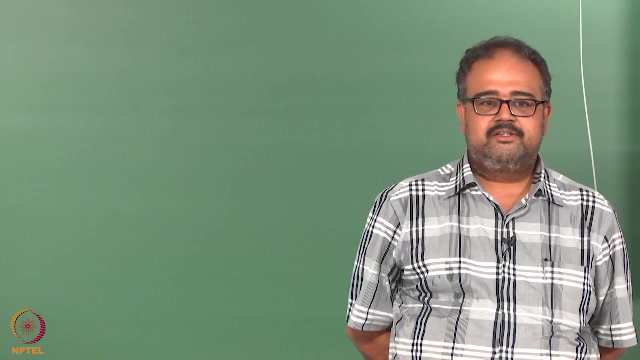 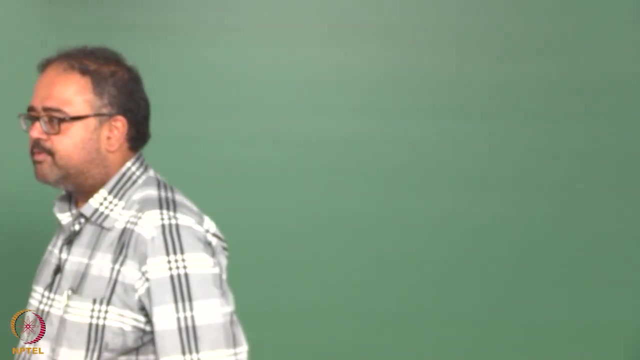 So how would you model this problem? so what are the states and what are the actions? what should be the reward? reward seems to be easy, right. so well, what you wanted to do, you wanted to gather cans. so whenever it gathers can, whenever it gathers a can, you give it a reward. 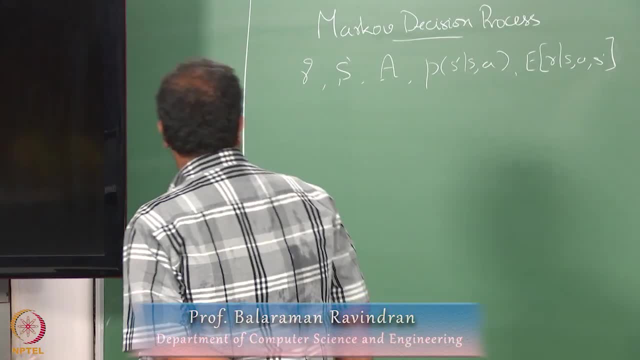 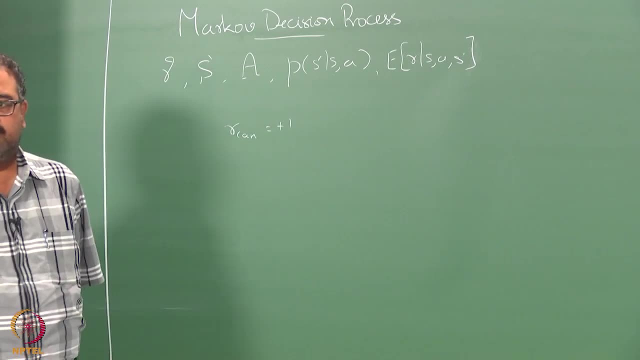 right. So, whenever it gathers a can you give it a reward of plus 1, right? So- and I am going to call this R can plus 1, right then, what you do not want it to do, you do not want it to run out of battery. 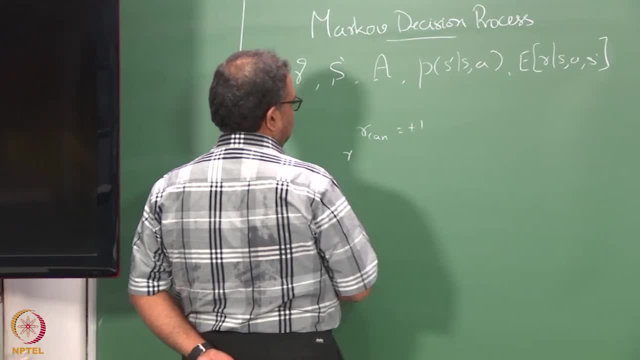 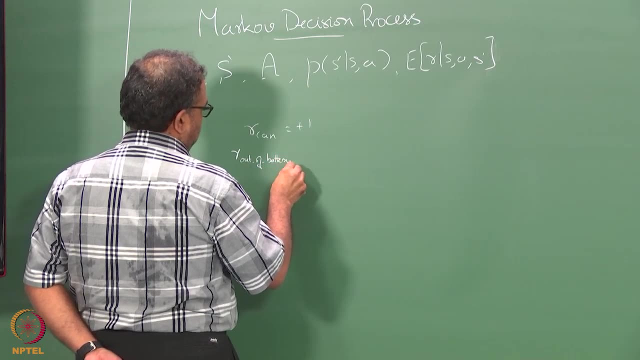 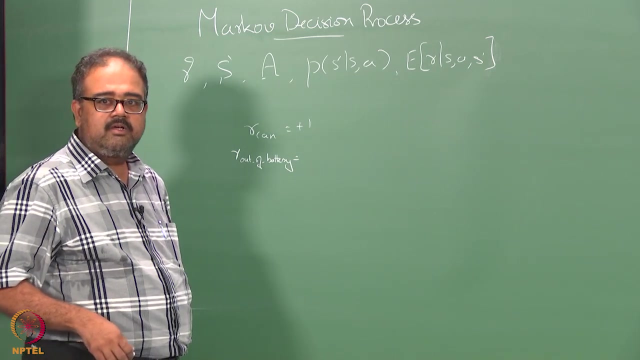 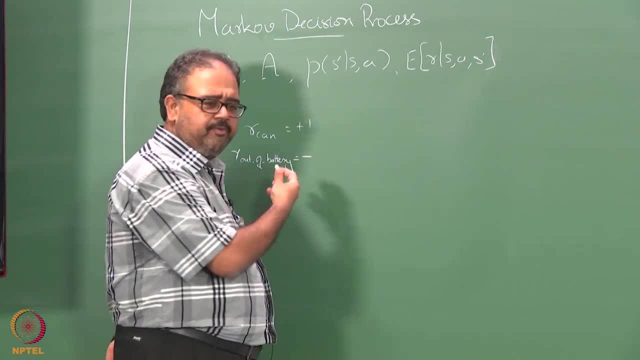 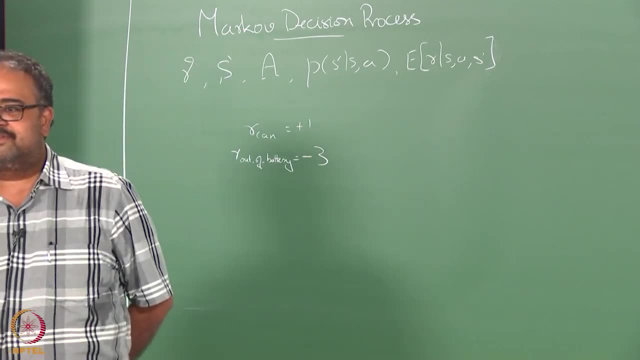 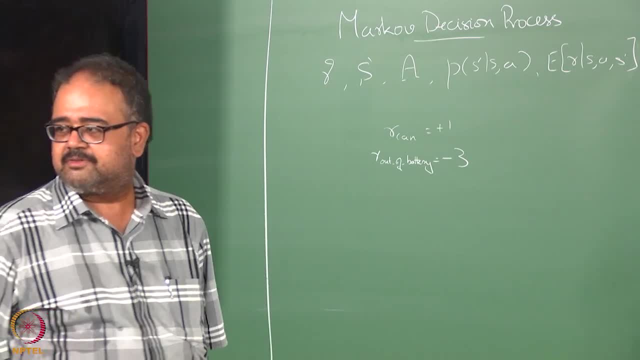 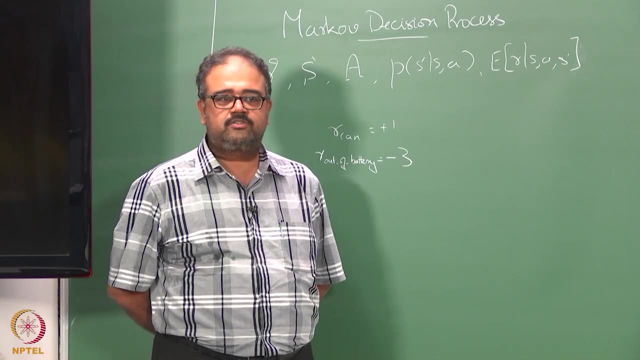 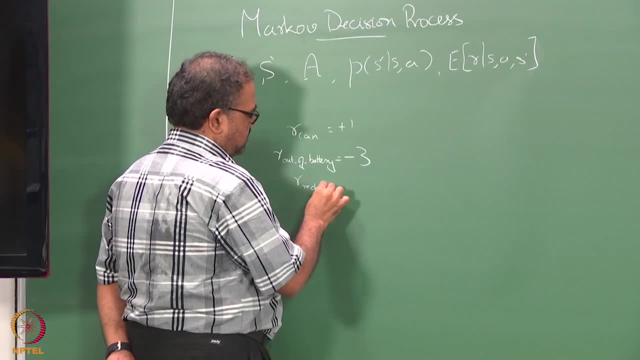 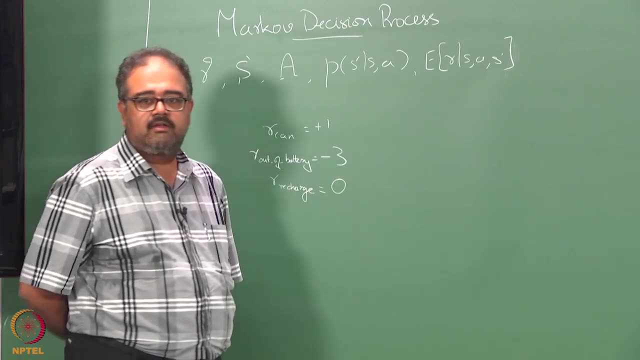 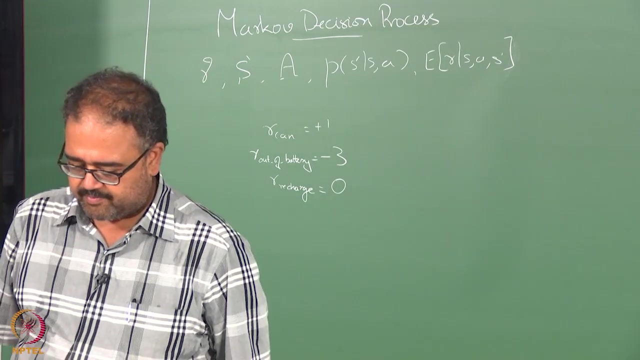 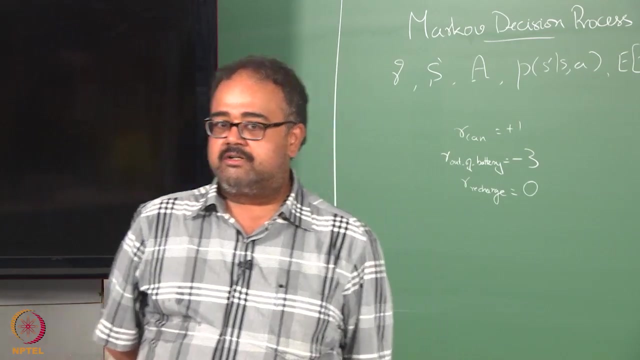 it a positive reward, or why does no reward make sense? it will give: yeah, just the heck for heck of getting that reward. it will get recharged, right, but then recharging is also good. we want to convey the fact that recharging also good, so it is better than running out. 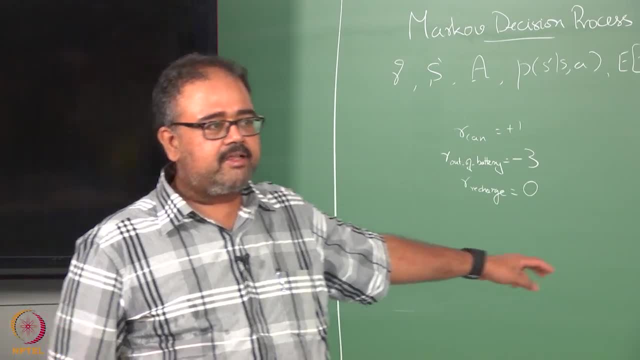 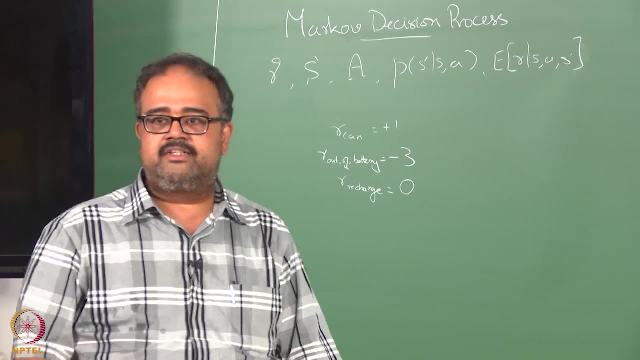 of battery and if you recharge, you have the potential for getting more rewards in the future, because you go out and seek more cans, right? so that way you have an indirect incentive for recharging because in the future it allows you to do something better, right? if you just 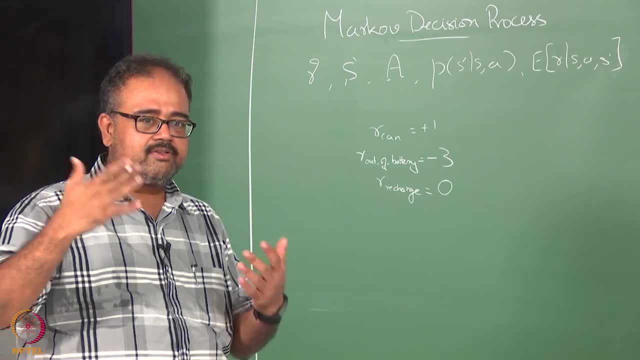 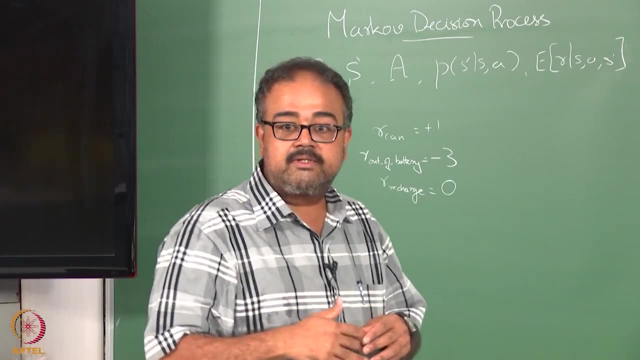 look at the immediate reward, it looks like a bad thing, but if you think about it, so in the future you are making it more attractive for recharge. I mean, if you look at the future outcomes, recharging is also very attractive. okay, Sir, can we scale it as in: if it is very low, if it is below a threshold or something, what? 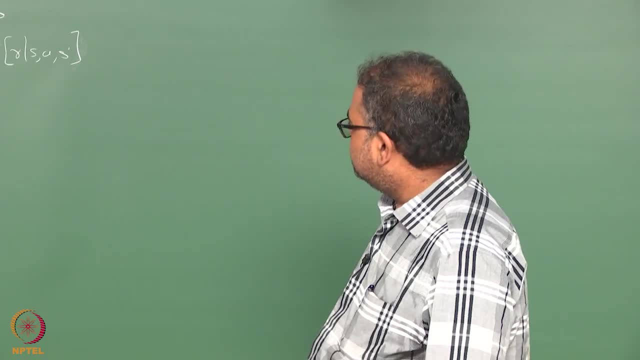 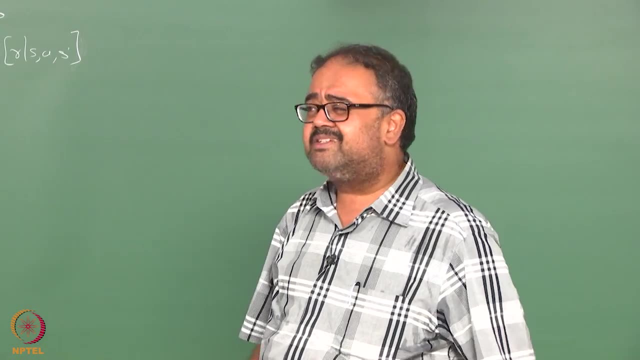 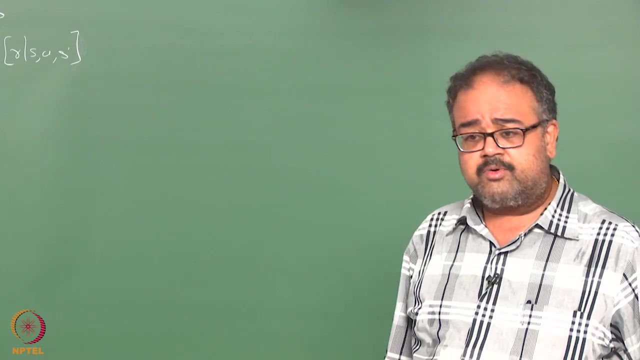 is below a threshold, if the charge no, no, this is not. this is if you think about it. this is more to do with actions or something, yeah, kind of with outcomes. yeah, battery levels. you could, you could make it all the more detailed. you can make it as detailed as you want, right? 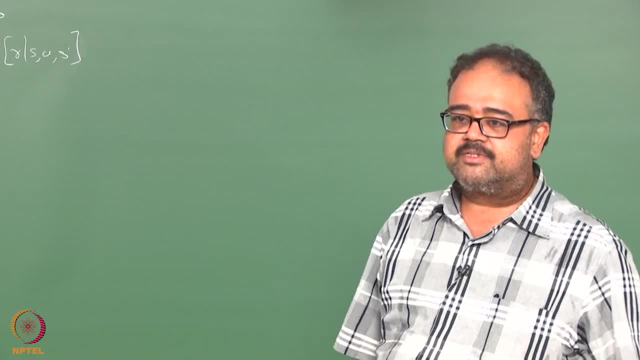 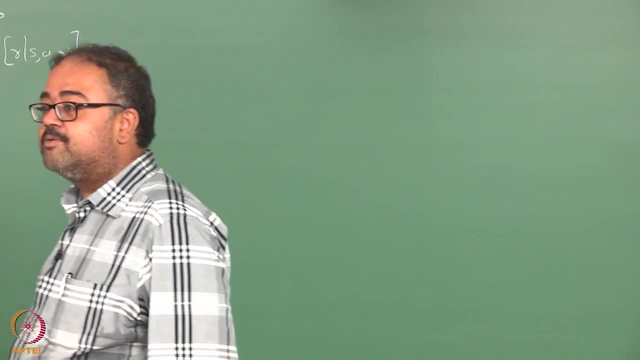 now. now comes the crux. how detailed do you want to make the representation to be? Do you want to make it a real number saying, okay, how much battery charge I have? you could get a continuous state then, right. so what do you want to do? you want to do some kind. 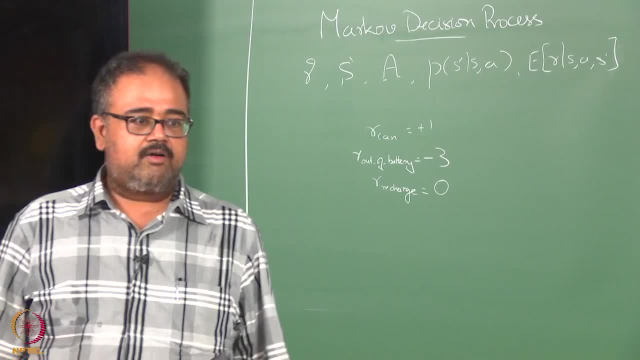 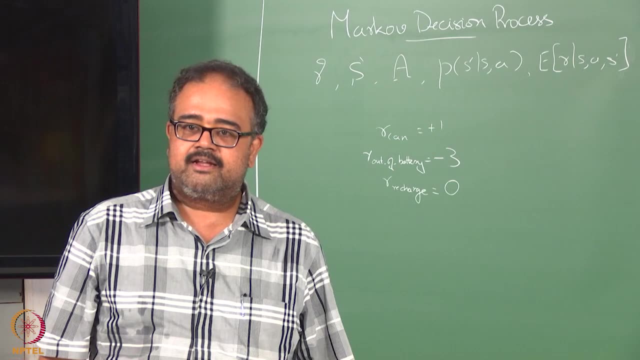 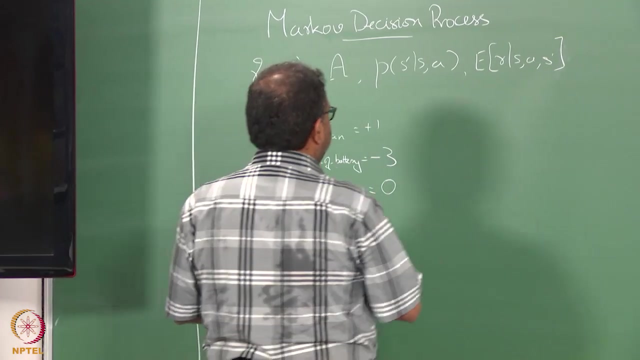 of discretization right. so if I want to do a discretization, so how do I discretize? that brings us to another question that completely we forgot to answer that question: what is the state? battery charge level should be the state right and then anything else is the? 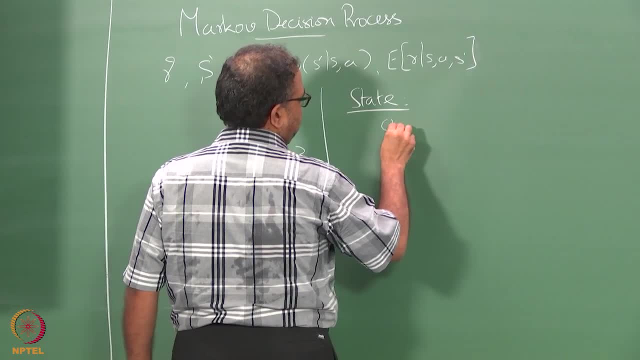 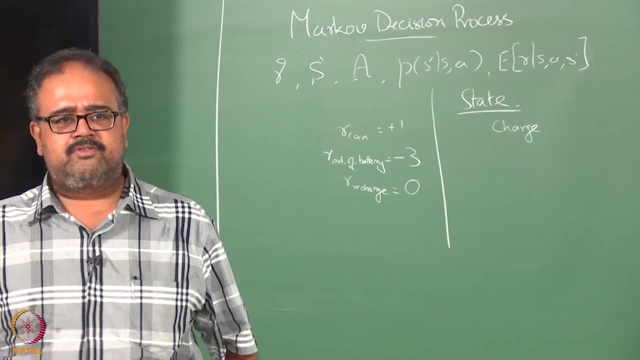 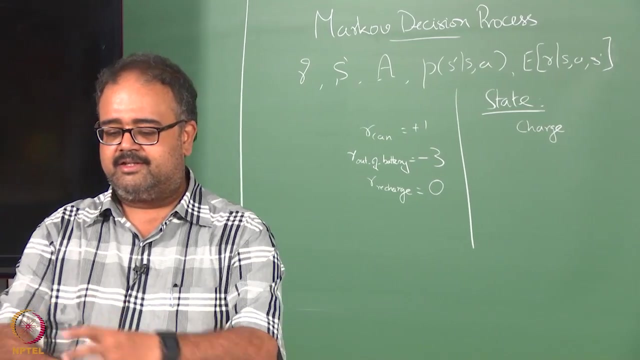 number of cans. No, let us just assume that magically it takes a can and transports it to- yeah, but that is an interesting thing. if it has a finite carrying capacity, then you probably need to throw in how many cans it has, and so before it has to make a trip to the dumping ground or something, 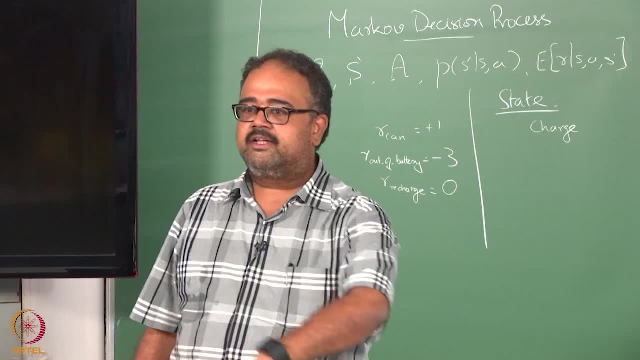 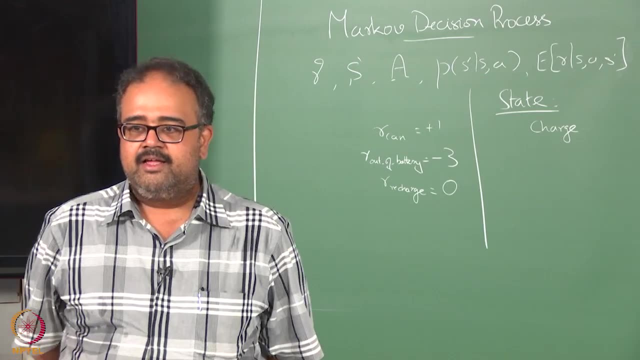 like that. so let us assume for the time being it is: as soon as you put a can into that, there is a teleporter that takes it to the dumping ground, okay, Or the bot has an infinite carry. I am just trying to make the problem simpler, right? if? 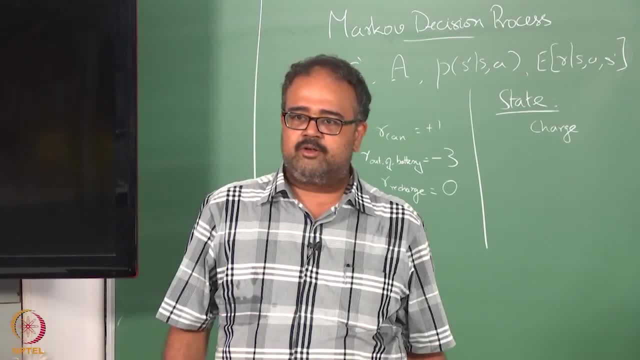 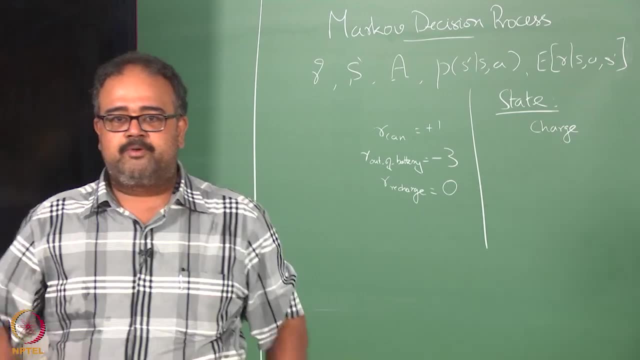 you want to make the problem more and more realistic, right, you will have to think about a whole bunch of other things, right? for example, I am kind of making it at a very, very high level. I am not talking about the pose, and I mean the pose of the robot, right, the velocity. 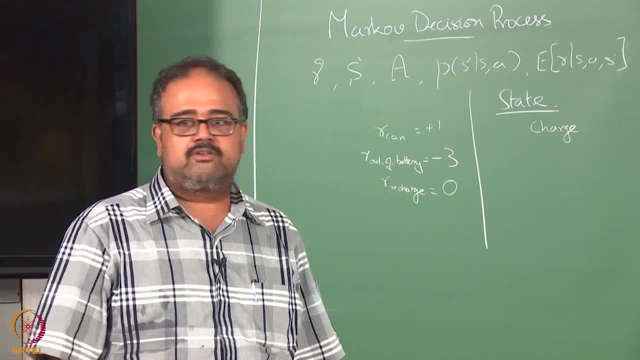 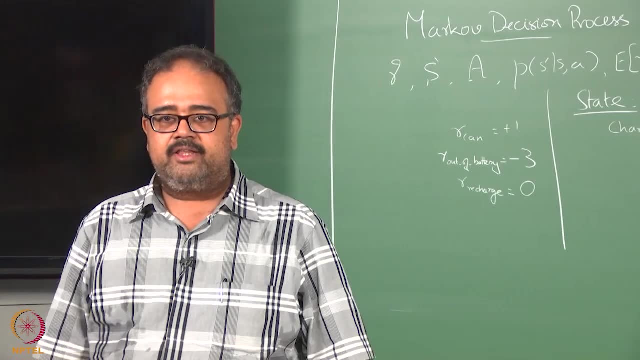 which the bot is moving. so all of these things you need, right? if you want to actually going to control the bot, right then, just assuming all of those are somehow going to be magically taken care of, right? So we are just assuming that you are only worried about the 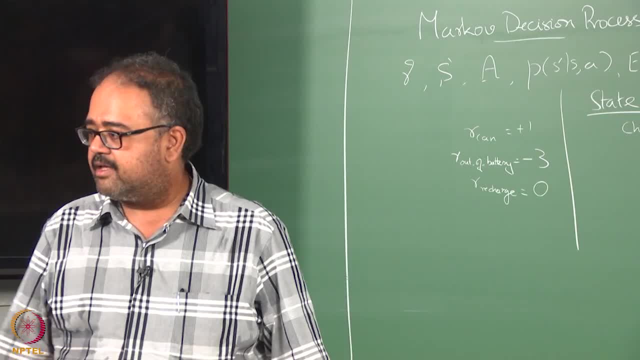 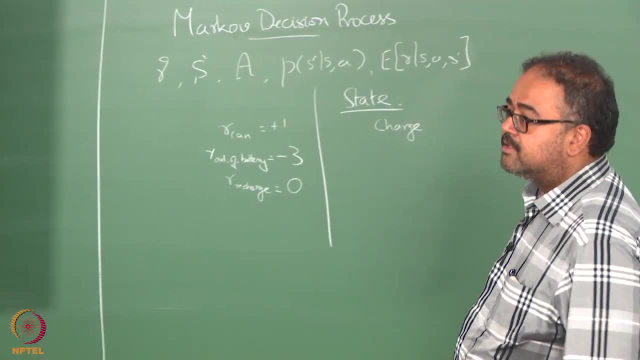 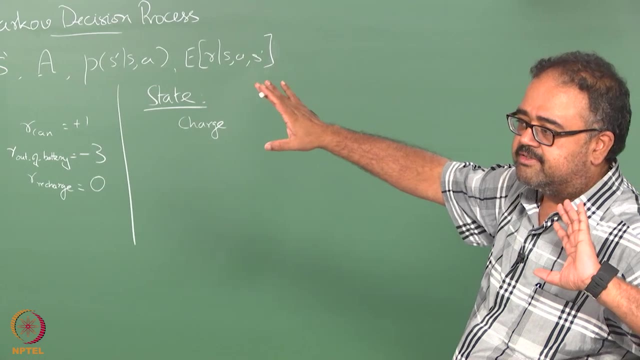 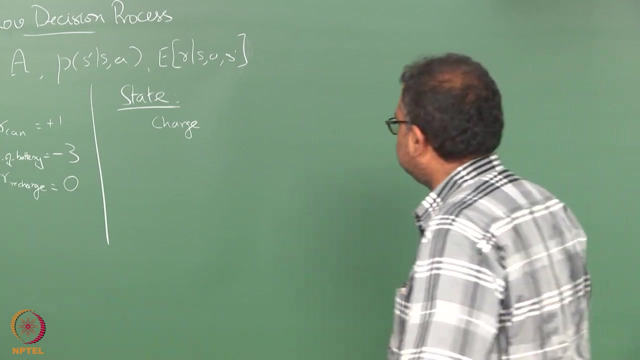 The, The charge of the bot, right, yeah? yeah, we have been talking about only discrete states and discrete action so far. we have not talked about continuous states and continuous actions. but you have continuous state, continuous action, MDPs. okay, so the state is going to be the. 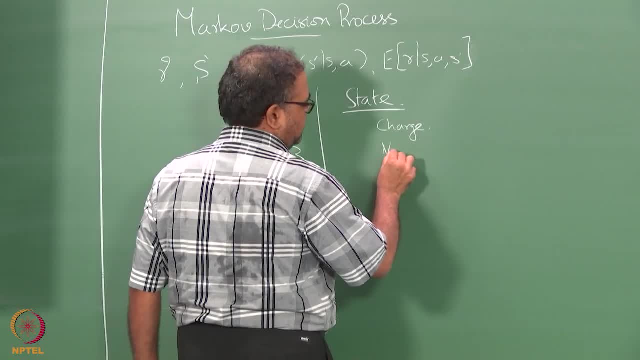 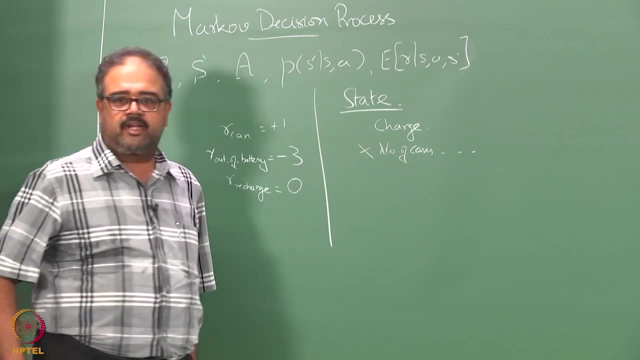 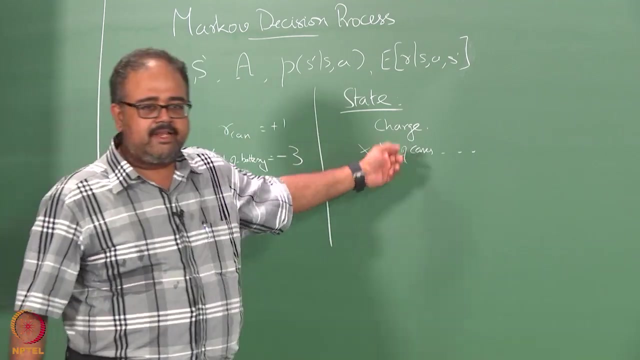 charge right And possibly number of cans Right and other things. but for the time being I am just going to say I am not going to care about all of that. we will just look at charge. just to keep it a simple, simple example right. I am also keeping it in sync with the book, so and again. so what do I do with charge? I 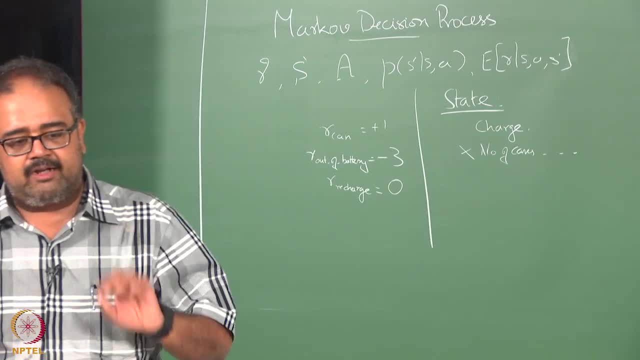 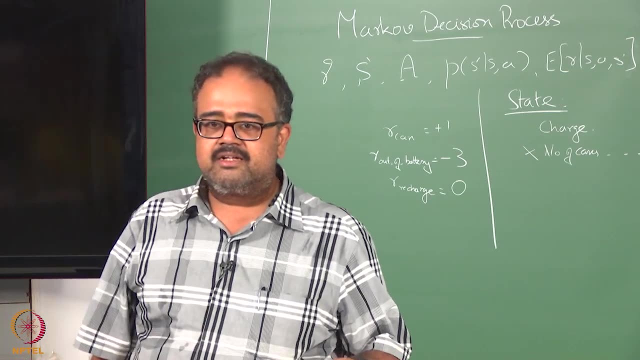 can treat it as a number, in which case I will have to figure out how to handle a continuous value, right, or I can start discretizing it. so how will I discretize it? Yeah, Yeah, Yeah. So how will I do that? because I am not going to be able to do it right, because the percentage 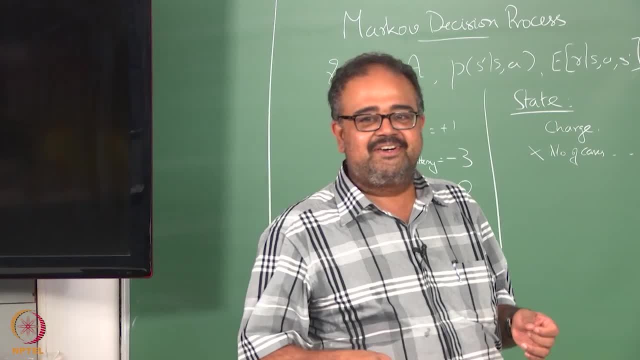 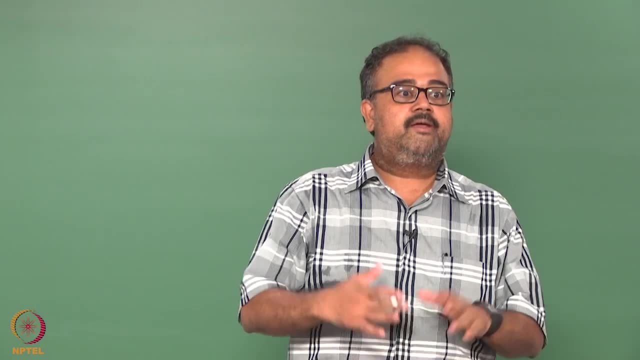 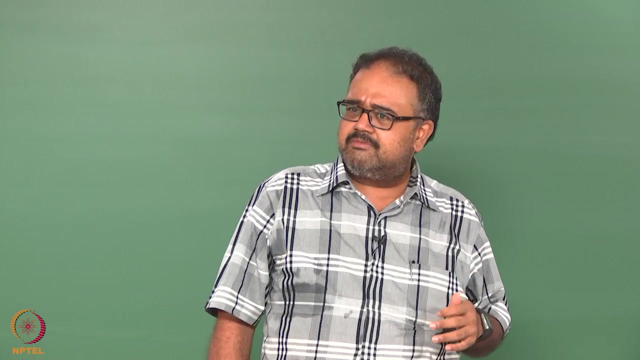 is also not a discretization, unless you round it off. okay, so yeah, so you could do something like that, or it could be even more aggressive. right, I could do low, medium high? right, and if you really stop and think about it, when would you if I say, if I do low, medium high, 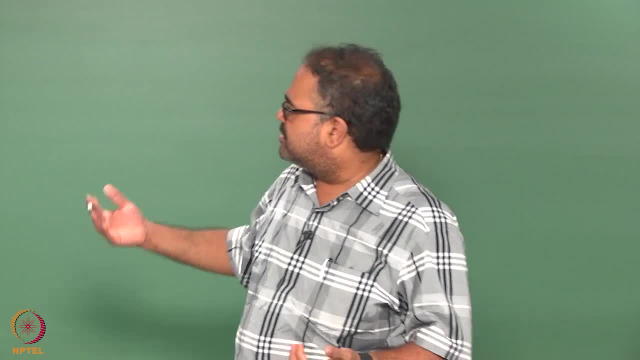 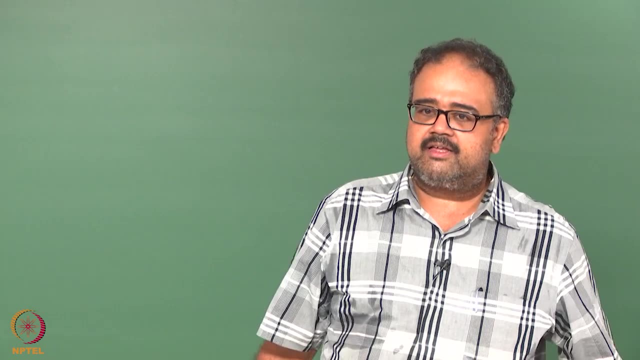 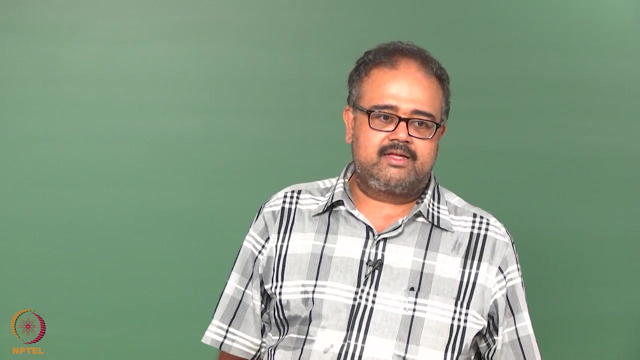 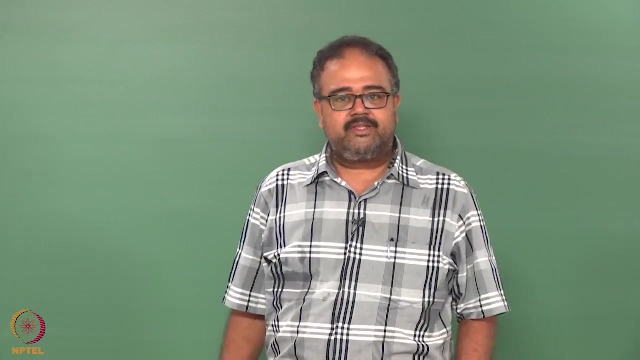 or something like that. when would I actually change my decision about charging versus not charging? it is only when I low, right, Yeah, even try operating with high and low and or sufficient and low, or whatever is it. mid is also problem, yeah, great. so I am not having my location at all here, right? so, assuming, 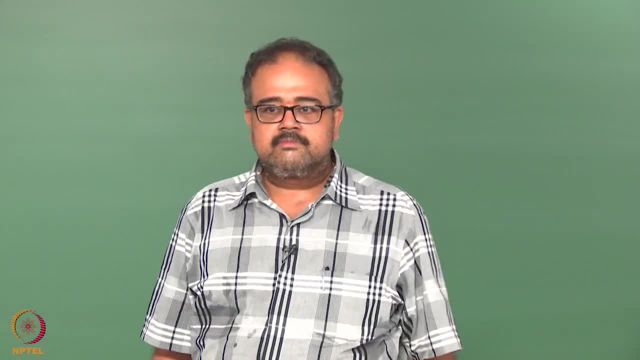 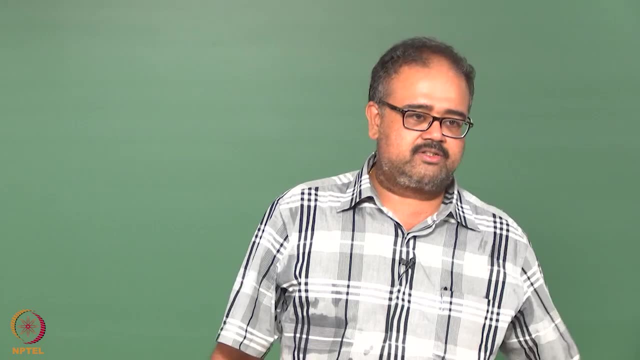 that there is always a convenient charging point located nearby. okay, so it is not like there is single base station. I have to go there. so as soon as I find out. okay, I am running out of charge. let us assume that as long as the battery is low, I can still get to a charging. 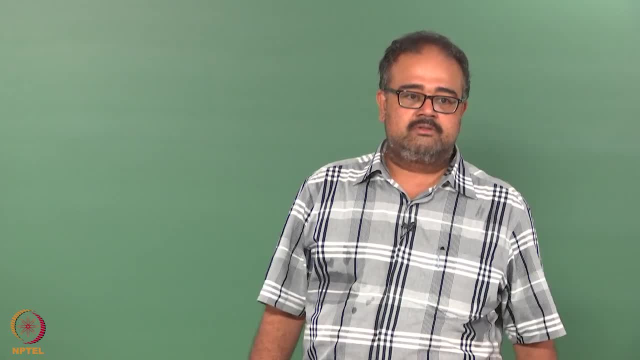 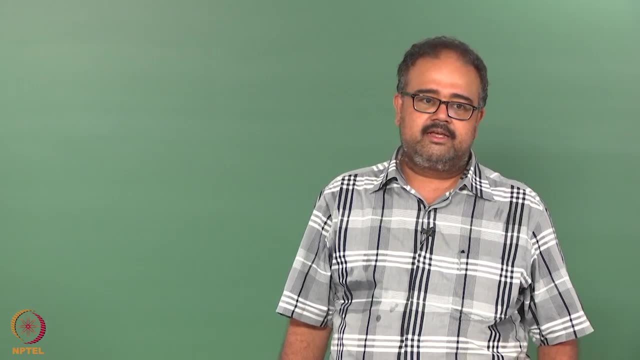 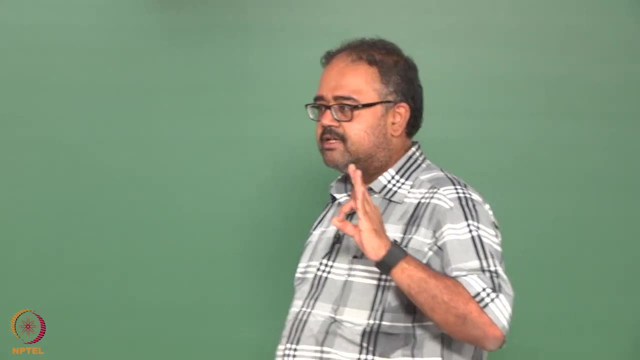 point. in fact, I am going to assume even something stronger so I could, with some probability, keep operating even if my battery is low, right, and I will still not run out of okay. the assumption I make is the following: whenever I say recharge, okay, I will have enough battery power to reach. 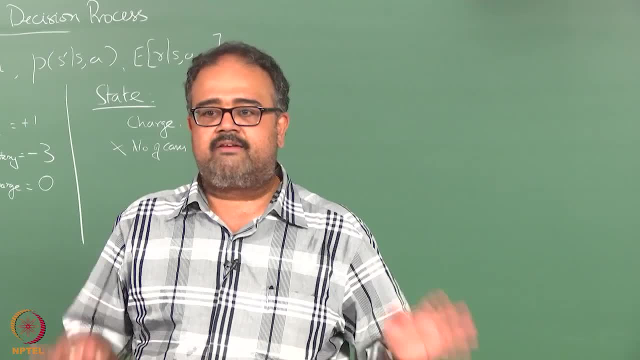 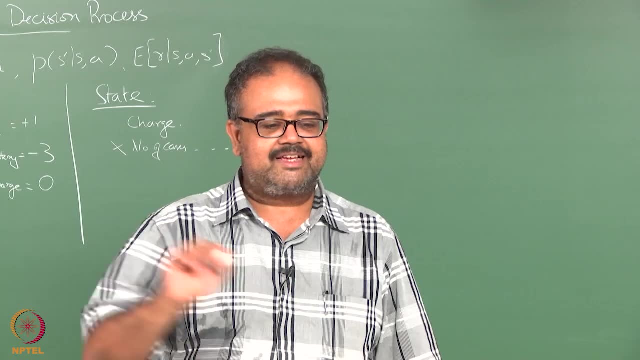 the nearest recharge station and recharge. so after I pick the option recharge, I will not run out of battery power. this is again a very simplifying assumption, right? this makes it easier for me For us to draw pictures, as I will do in a minute, right? but all the points that are being 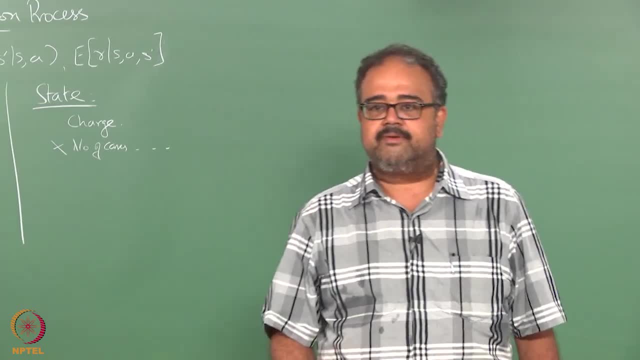 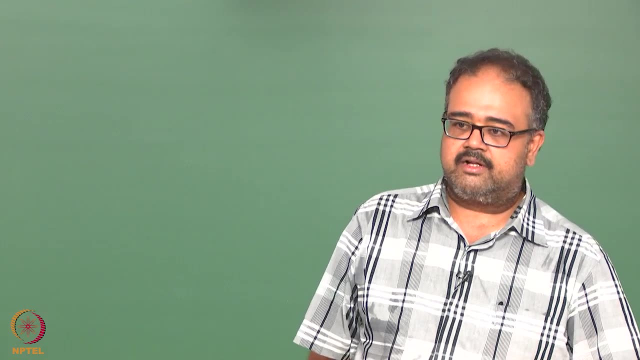 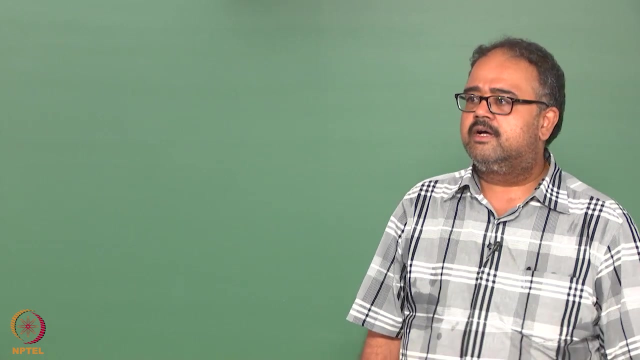 raised are very good points, right. so when you start trying to model a real system, right, these are all calls that you will have to make, right? so what is it that I would throw into my state? right, what is it that I can ignore? right, and so on, so forth, and yeah, so. 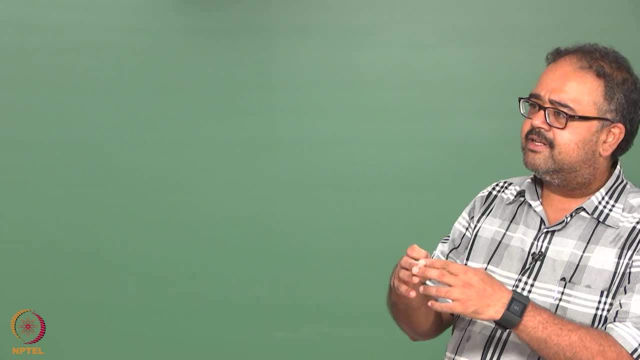 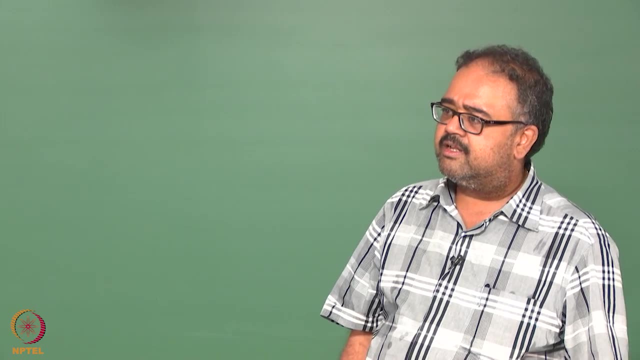 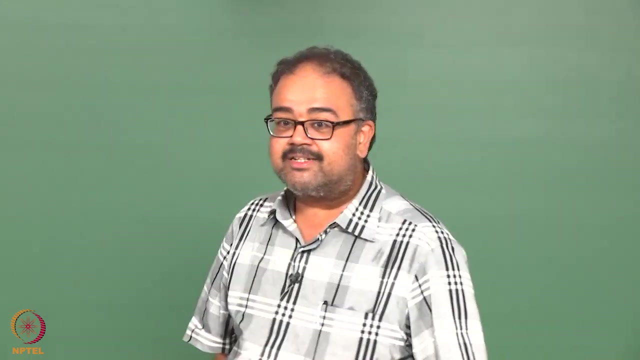 so, Pallavi, do you remember the homework assignment we are asking them? Yeah, the third one we are asking them. we are giving them a word problem and asking them to construct an MDP out of it. right, you think so? new assignment. third assignment: yeah, the one that was released today morning. yeah, it was released yesterday. then you are time traveling. 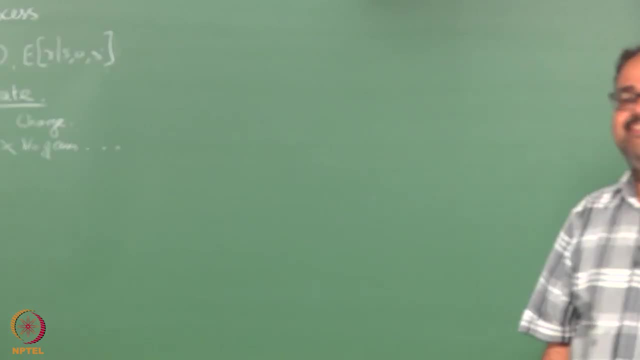 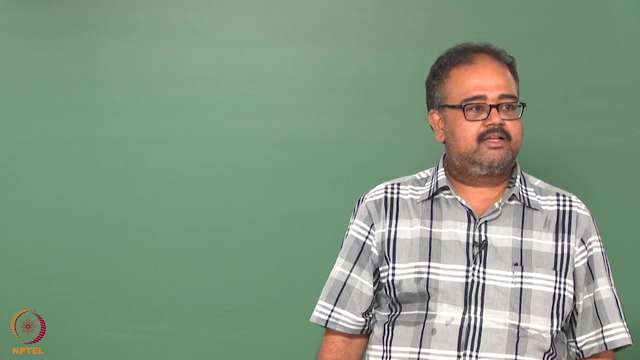 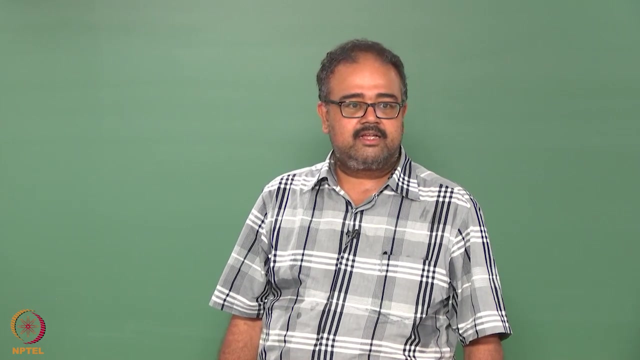 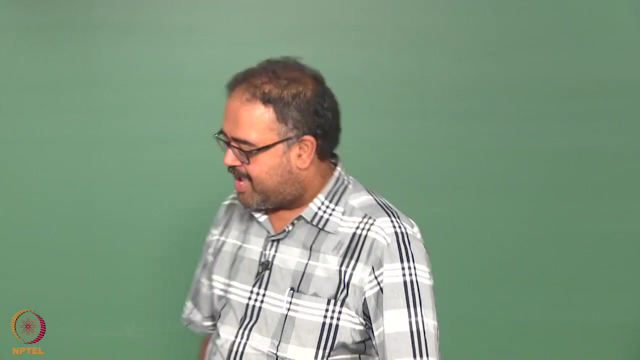 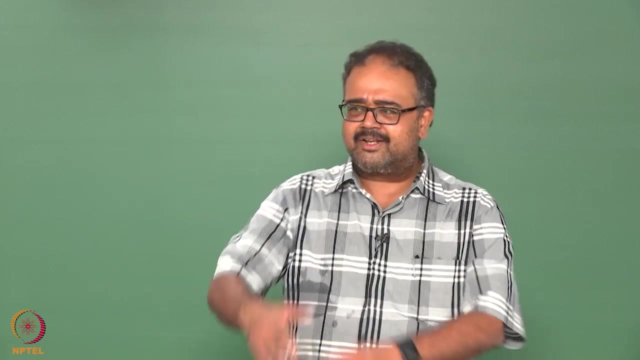 okay, yeah, it was released this morning. yeah, so the new assignment and it is due on Feb 14th. Yeah, Yeah, 14th. which is what? 9th Sunday, Sunday? yeah, well, plan ahead if it is important to you, finish on the 13th or, as it is more likely for lot of people, if you have nothing to do. 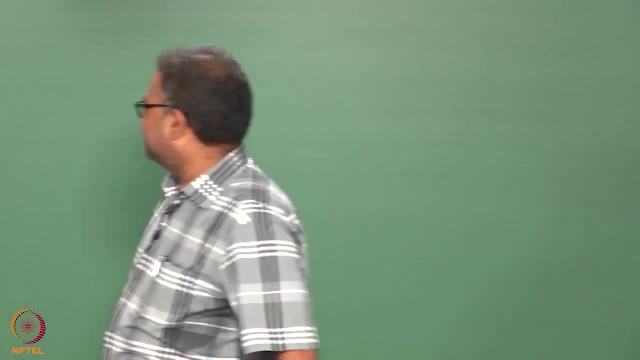 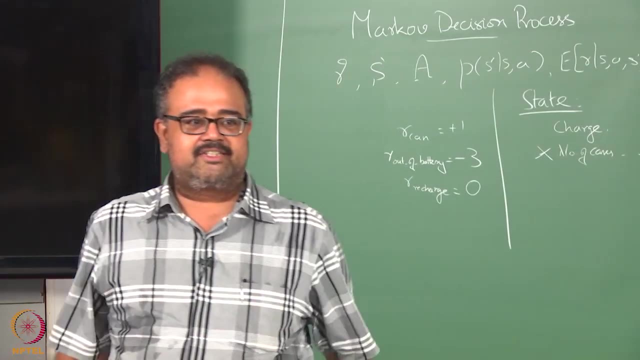 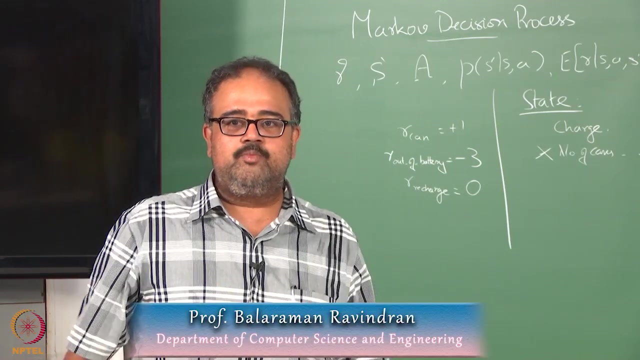 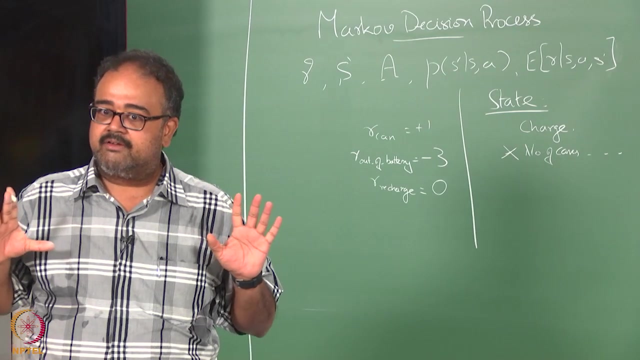 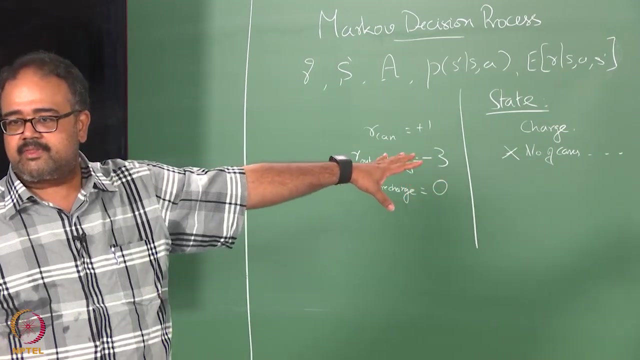 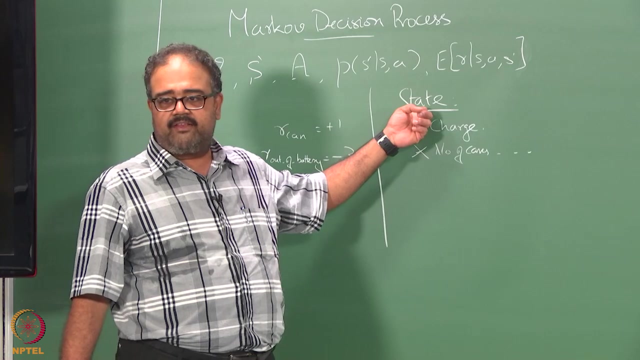 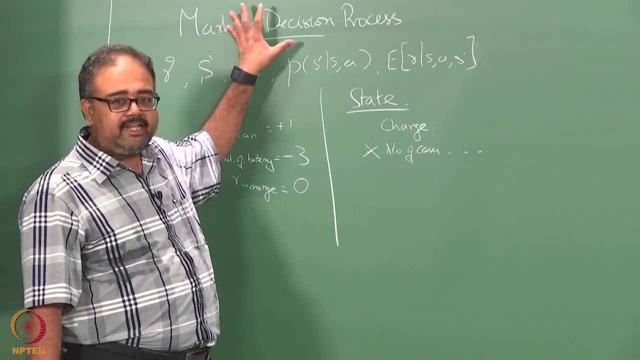 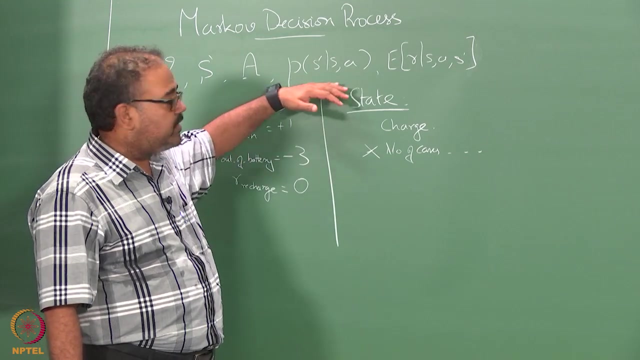 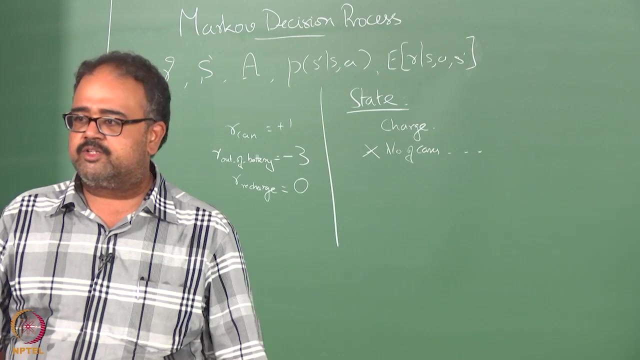 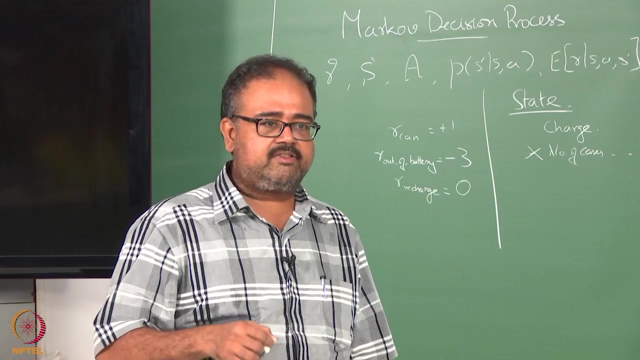 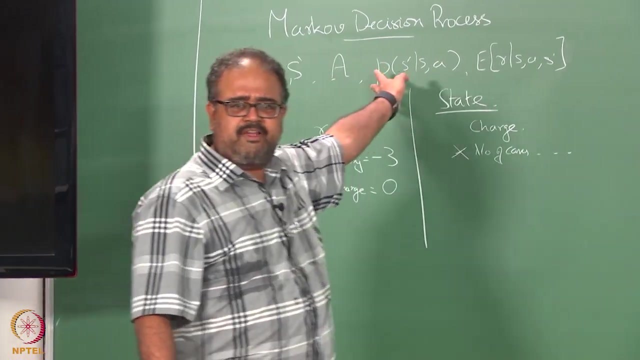 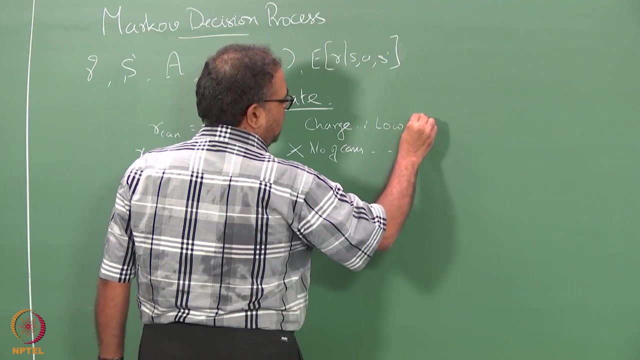 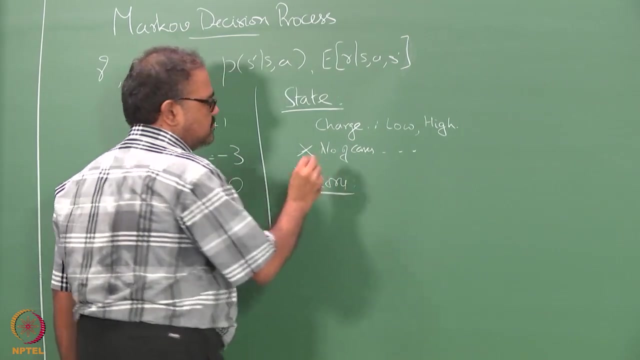 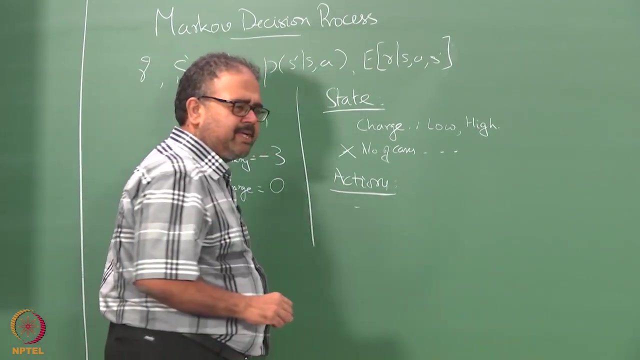 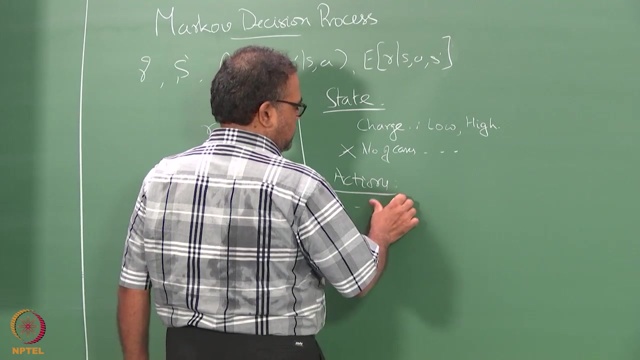 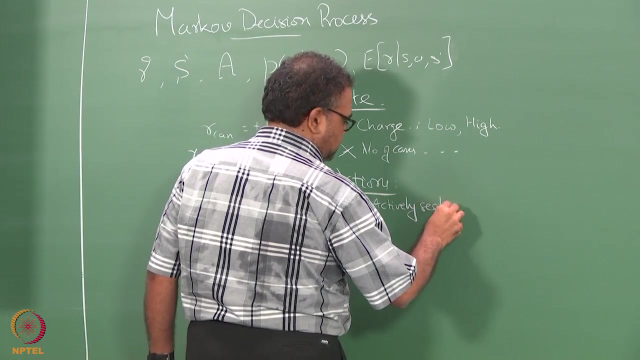 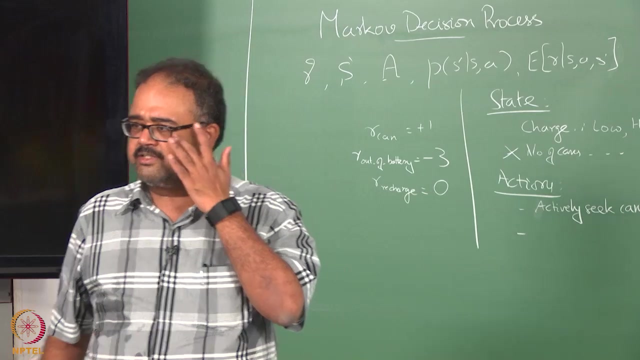 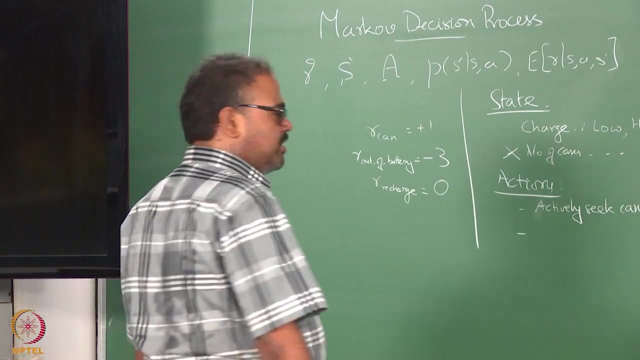 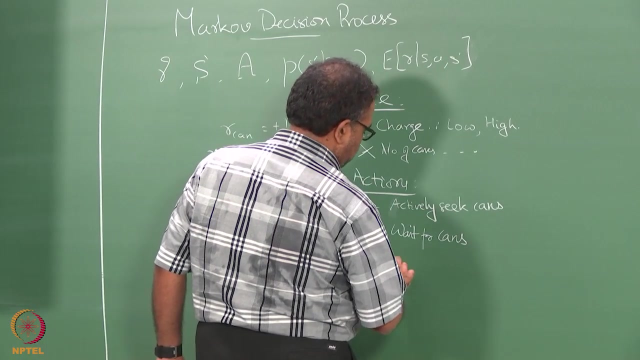 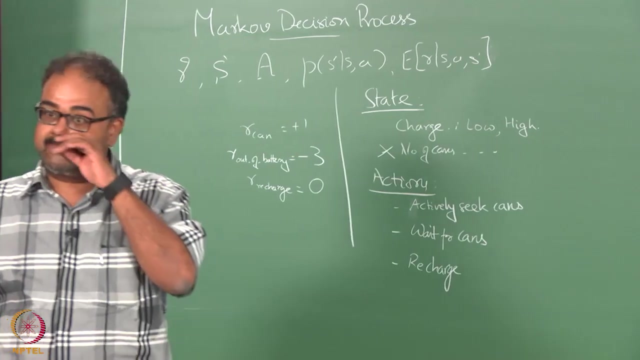 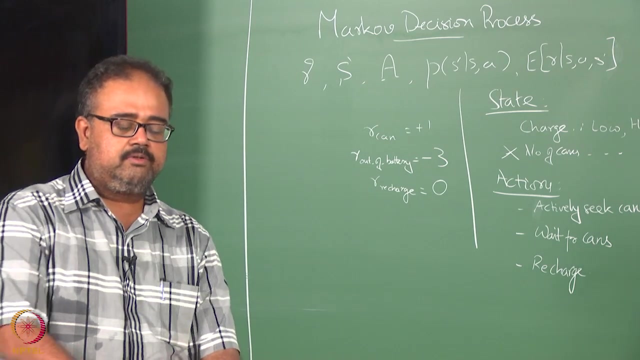 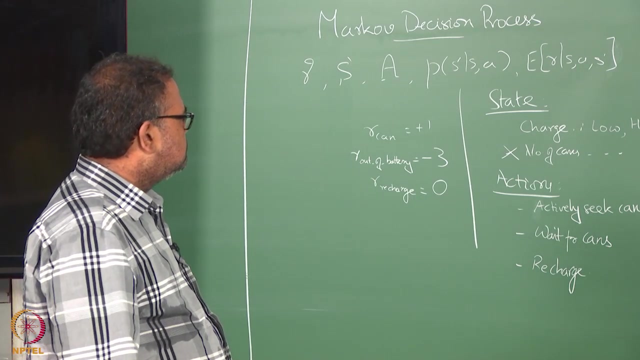 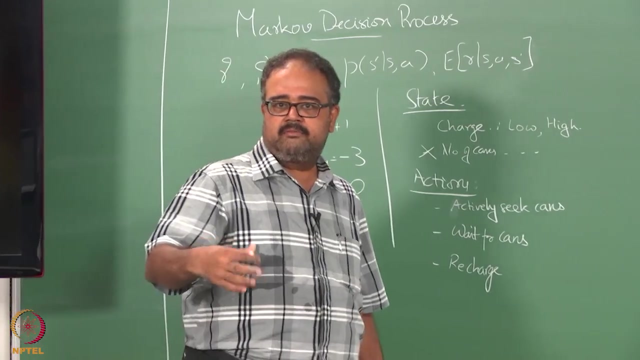 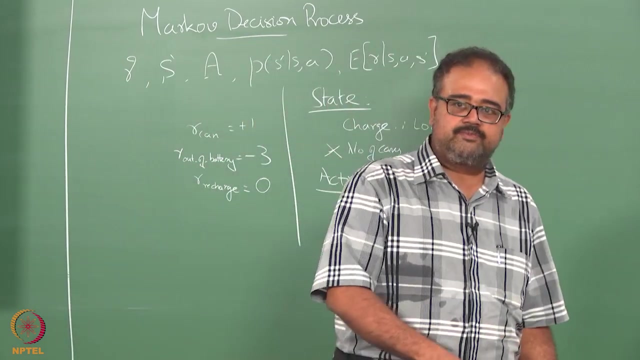 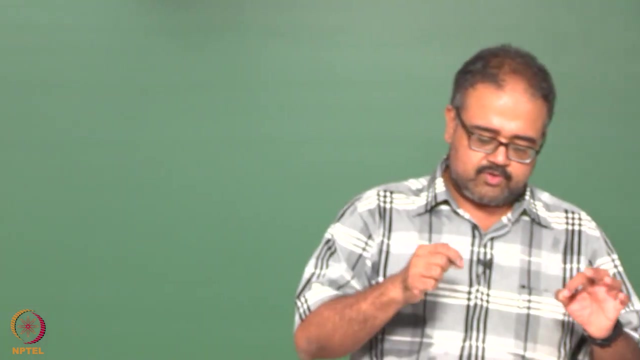 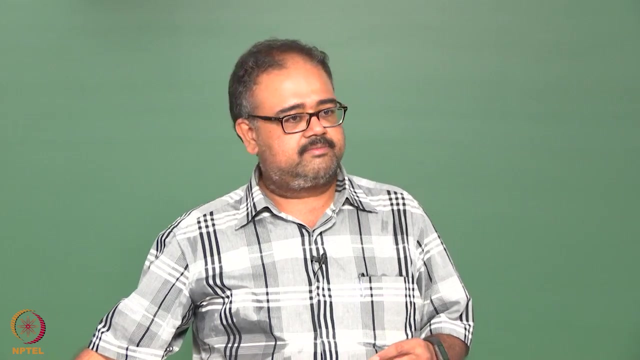 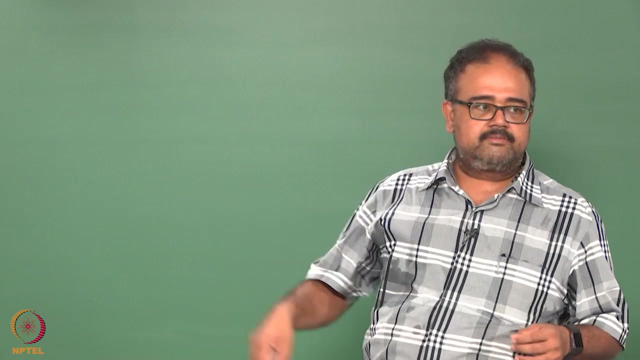 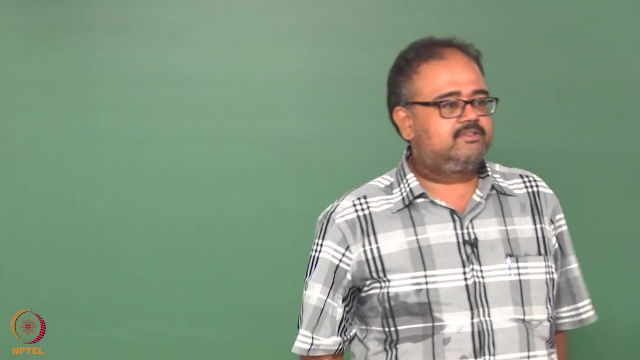 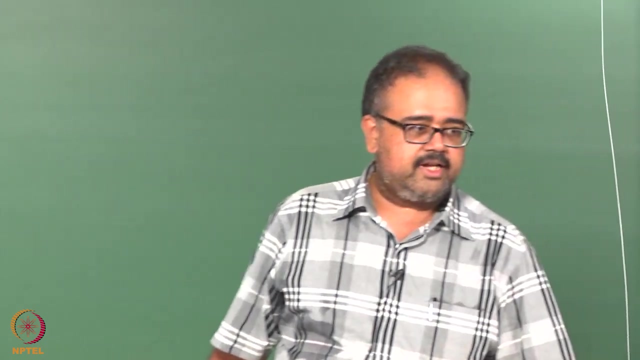 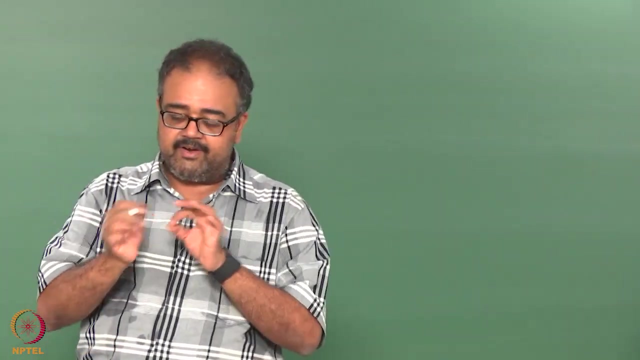 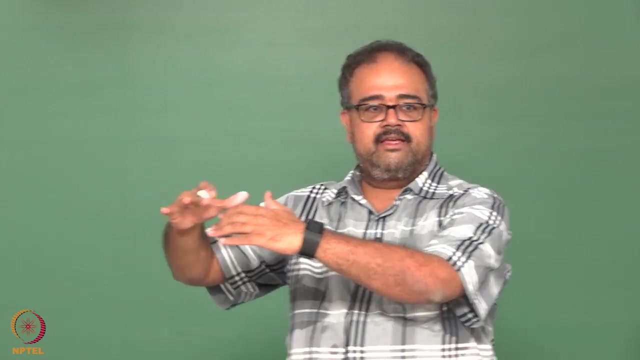 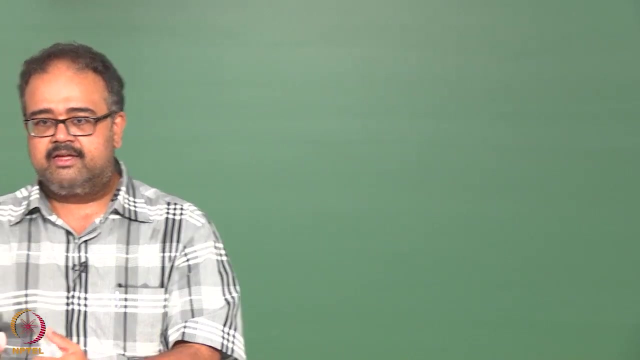 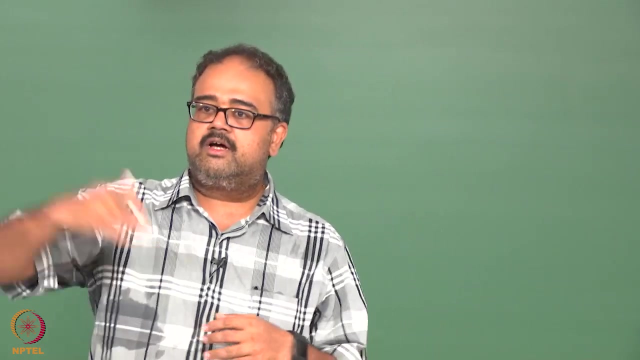 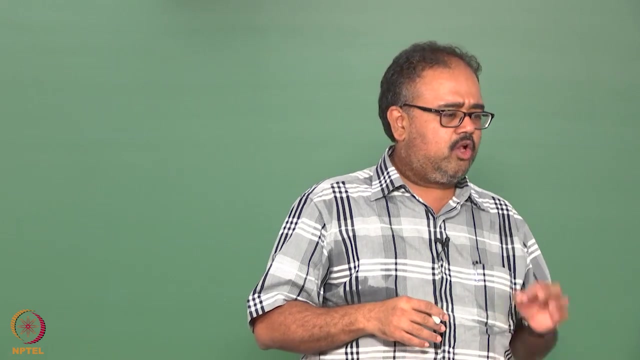 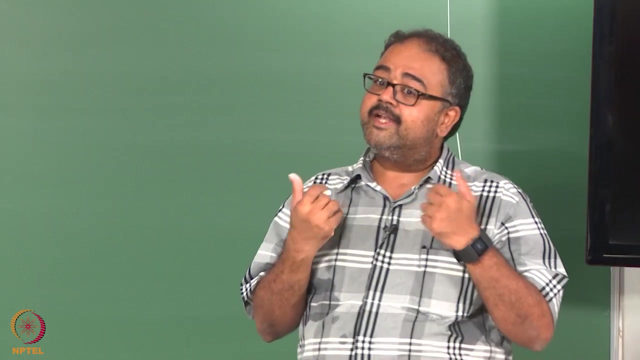 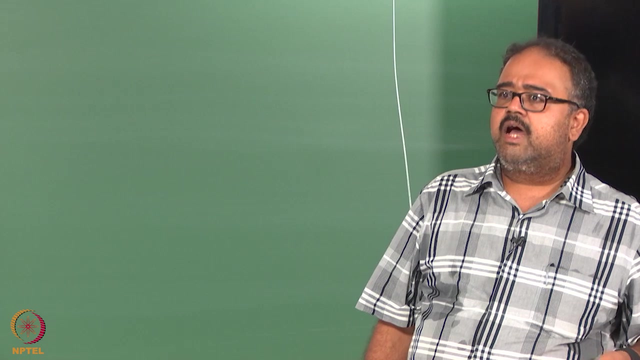 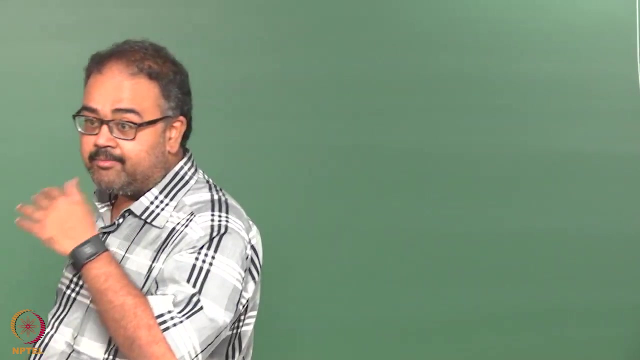 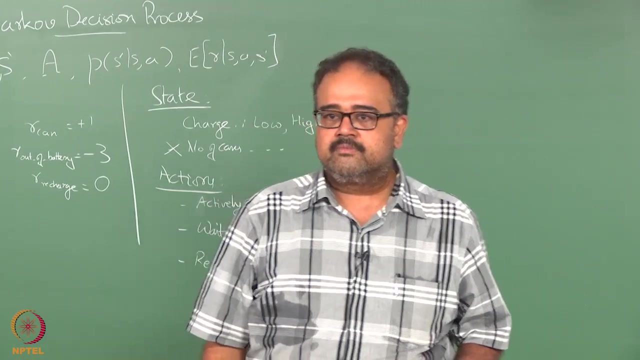 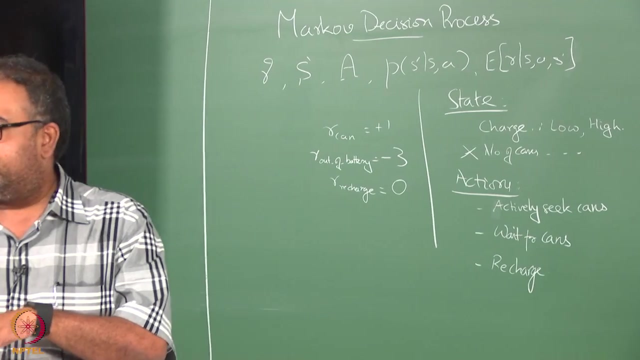 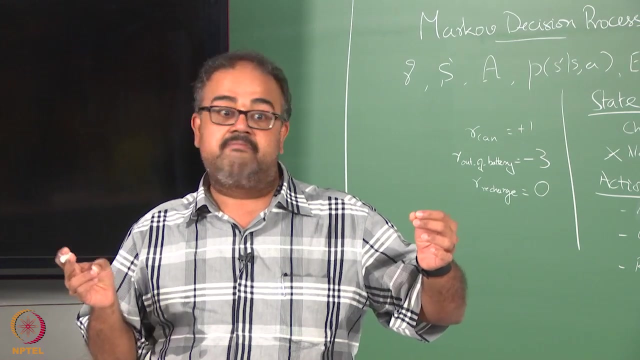 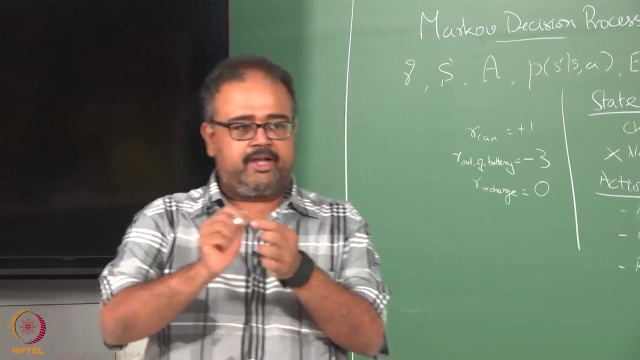 on 14th, only have a whole Now, at this point, if this is the action you are doing, this is so much power that you will consume and therefore the battery will go from high to low. 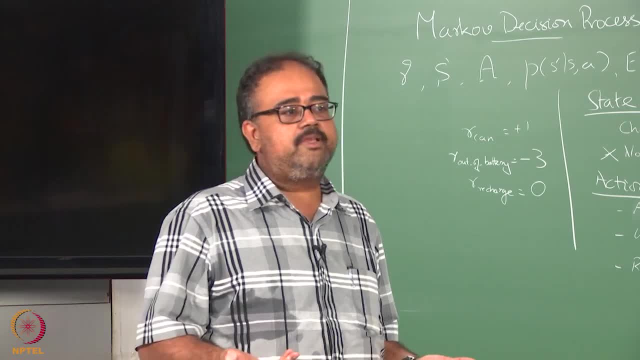 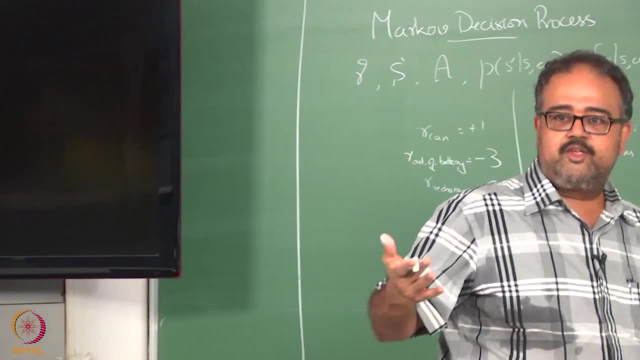 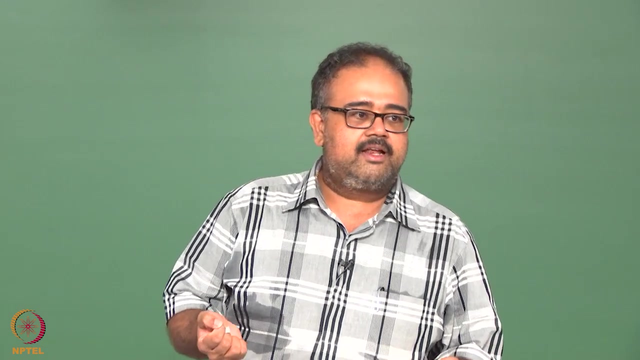 So I might be able to give that to you exactly. So inherently this might not be a stochastic system. I am only saying might not be, because people have worked with robots, so you know that you might specify as many initial conditions as you want. the bot will do what it wants to do. 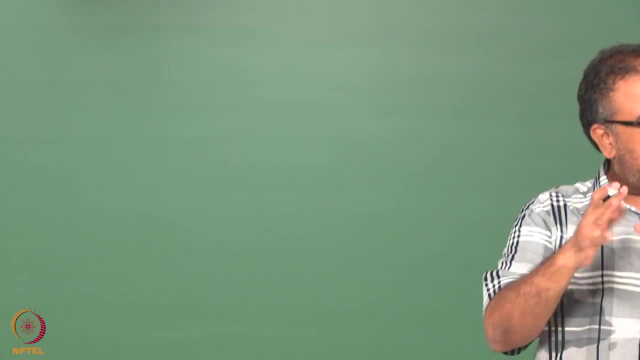 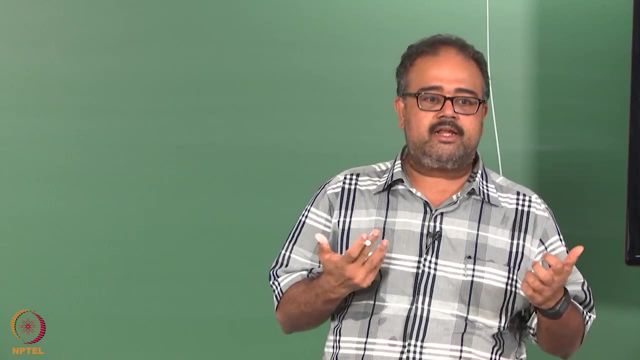 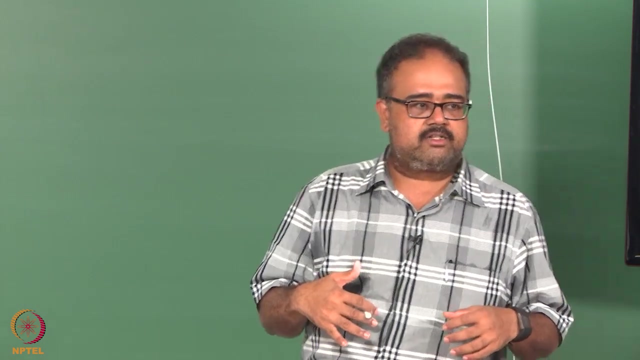 So it still be a stochastic system, but it could potentially not be a stochastic system if you know everything about the world. But we are making it stochastic by virtue of ignoring certain things that we could potentially know about the system, and ignoring this makes the system design a lot simpler. maybe we 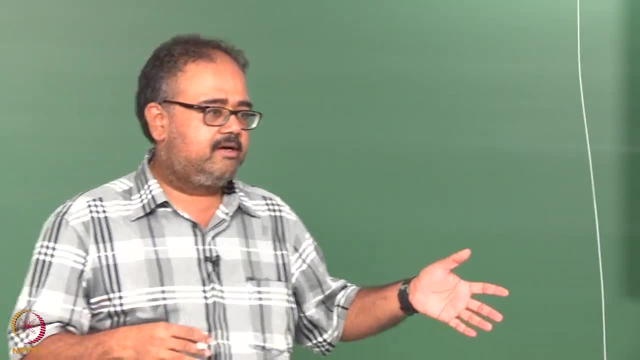 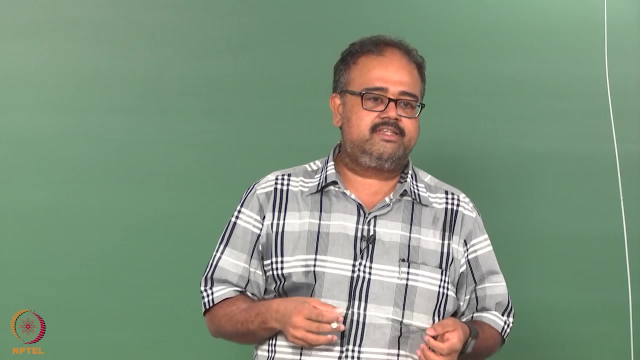 are giving up some things in terms of how optimal our solutions can be, but that is a trade-off that you will often have to make. So just the formulation itself is not an easy task. you have to think about it a lot to figure out what would be the right place to draw the line. 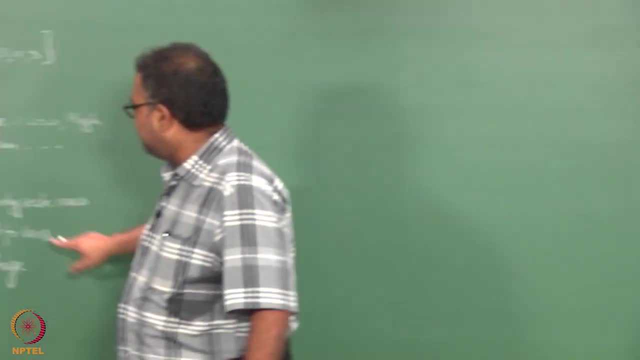 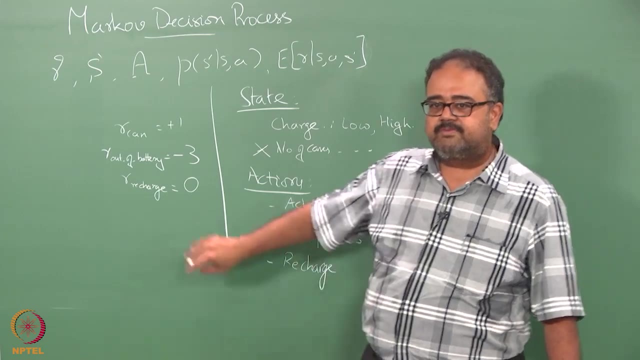 So these are the actions that we have to take So you can actively seek cans, wait for cans recharge. is there something else that we have to specify? So we have specified the stage, we have specified the actions, we have specified rewards for. 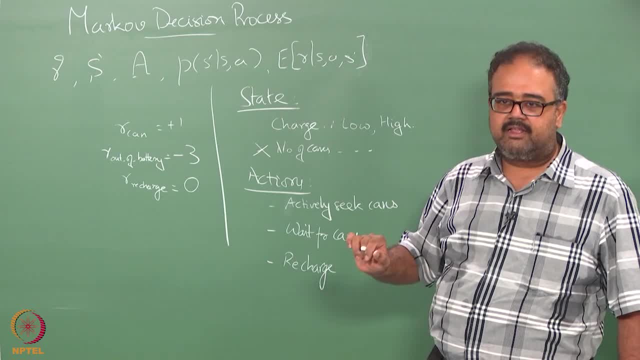 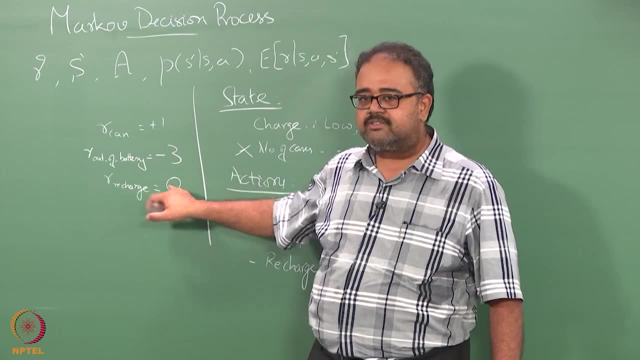 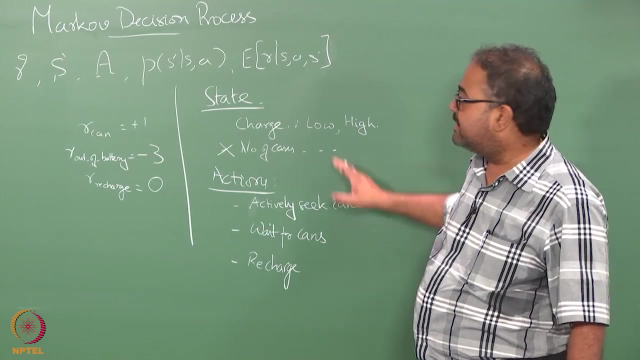 events. so if I collect a can I get a plus 1, if I run out of battery, you get a minus 3, then if I recharge, you get a 0, these are events that could happen in the world, So these are. so I have to relate this to the states and actions. only then I can tell. 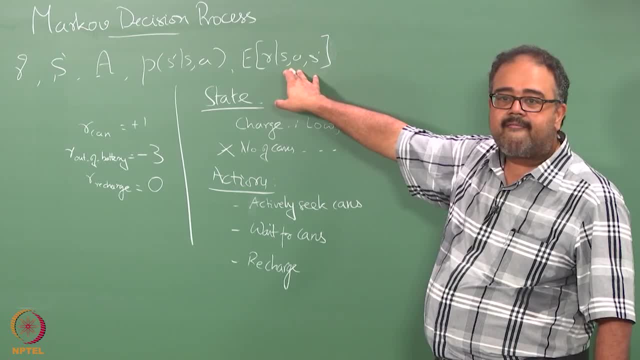 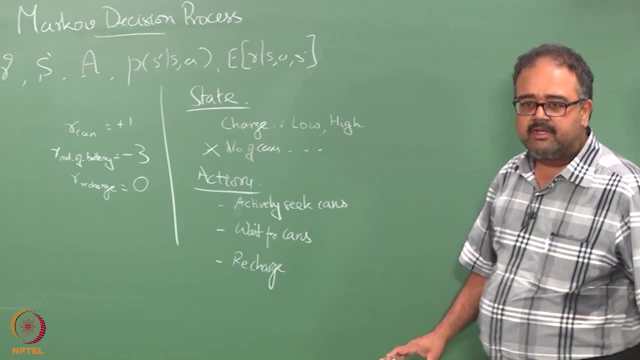 you what is the expected reward? We will not talk about time at all. so I told you for that, at least for the initial part of the course. we will not talk about time, that how long it runs. So what is it that we need? suppose I am actively seeking cans? what is the probability I will? 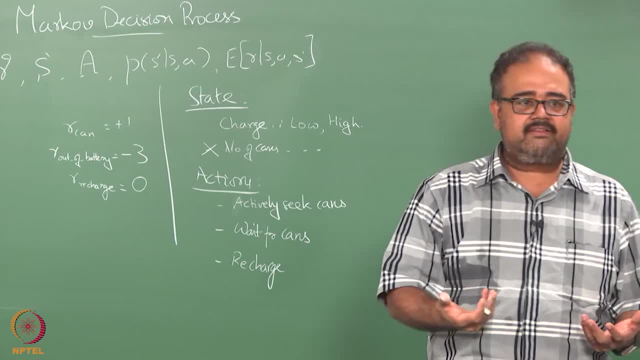 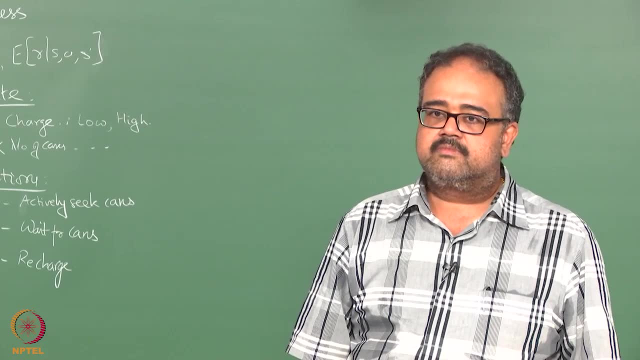 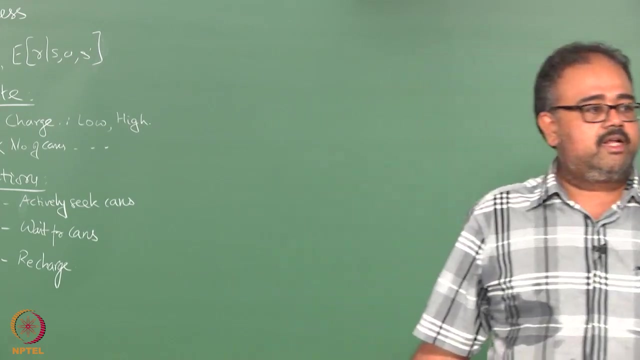 get a reward of plus 1?. If I am actively seeking cans, what is the probability that I will find a can? Correct, So I need to still specify. Yes, So I need to still specify that if I am actively or if I am waiting for cans to come right. 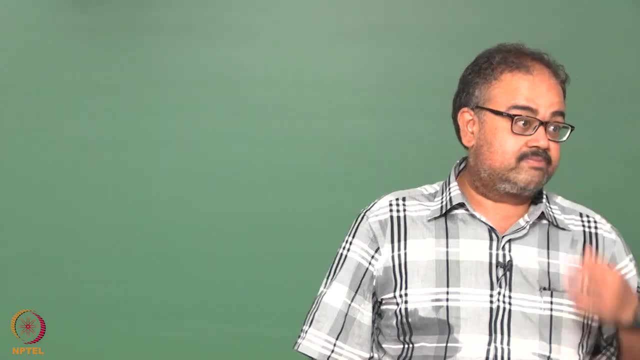 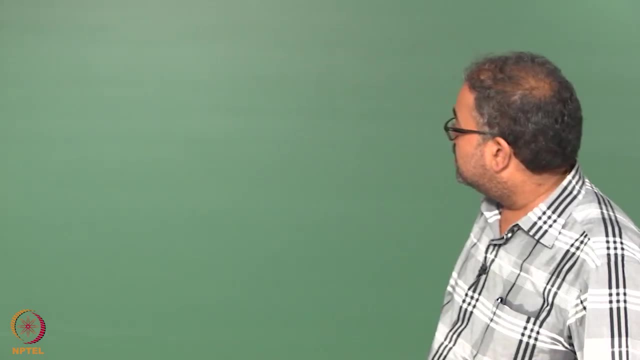 what is the probability that I will get a can? What is the derivative of what? Derivative of which one? If you are waiting for cans, there are no cans available, which means you no more actively seek a can. right? What is that? 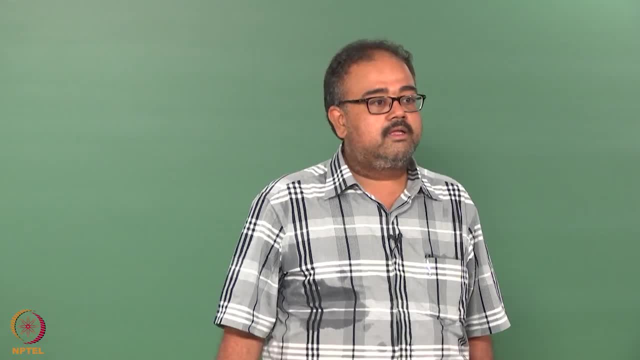 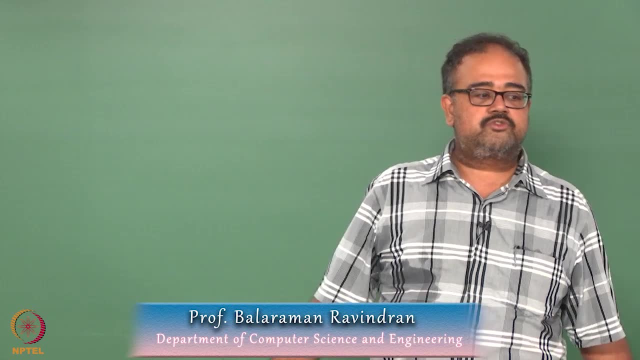 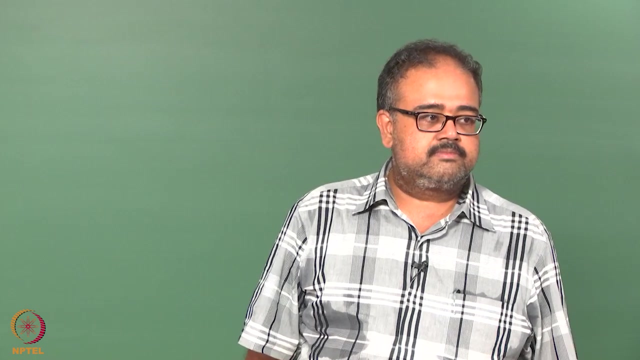 Which means you no more actively seek a can. Why? Because you are actively seeking a can, you decide that there are no cans available. I do not know why you chose to move from one to the other right. I mean, I could have just stopped seeking because I was running low on battery, right? 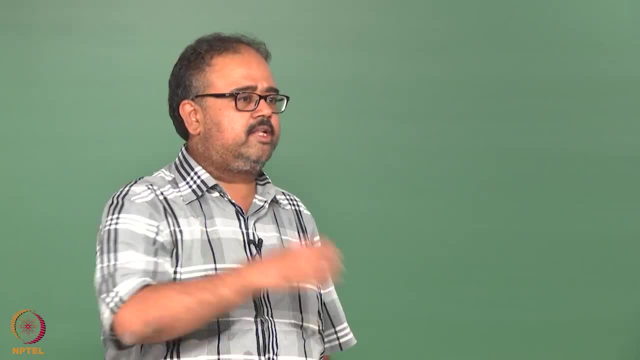 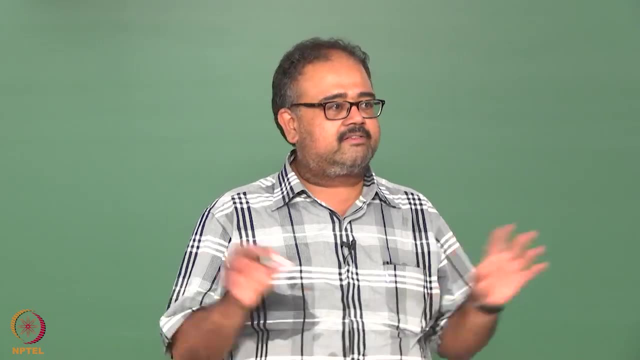 So if I am in some facility where people are just taking cans and throwing them in the dustbin, right, I might just happily go sit next to the can dispensing place and act as a dustbin, right. I will be happily getting rewards, right, I might not even worry about. 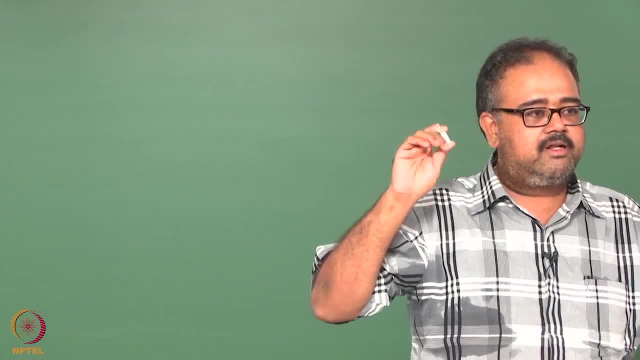 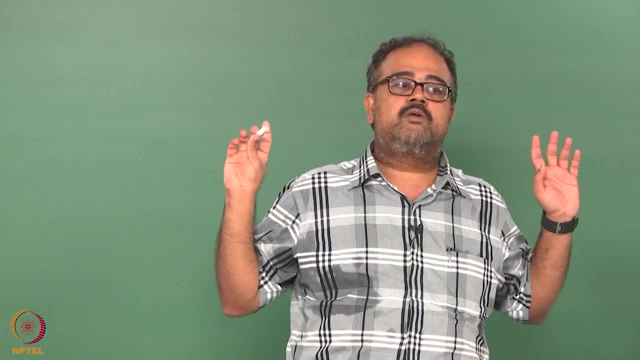 recharging or anything, right, so I might just choose to stop right. so it depends on that. depends on that. It depends on the kind of environment you are operating in, right? so even if I act as a dustbin, if do I get enough cans, then I might not want to seek right, so maybe there. 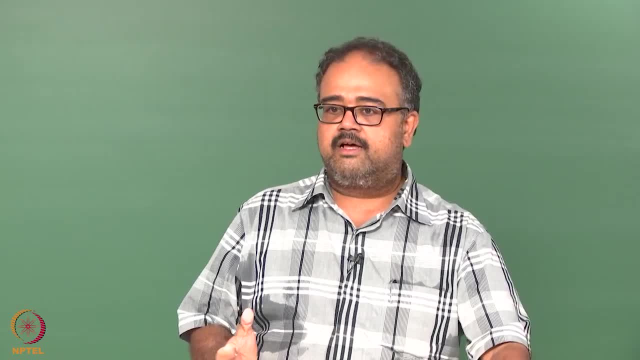 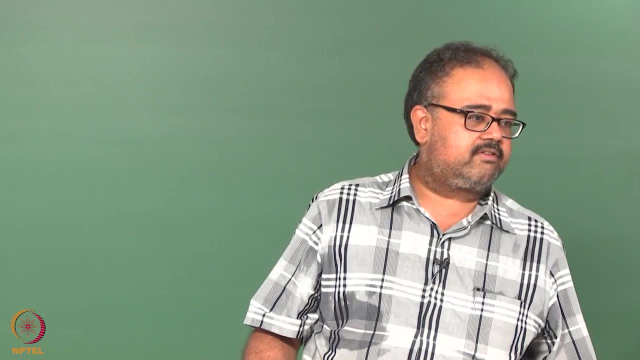 is some time of the day, maybe between 12 and 1.30 or something, lot of cans will come. if I just go stand outside the cafeteria, I do not have to actively seek cans. maybe after 1.30 I have to go around seeking cans, right? I do not know. it depends on the system. 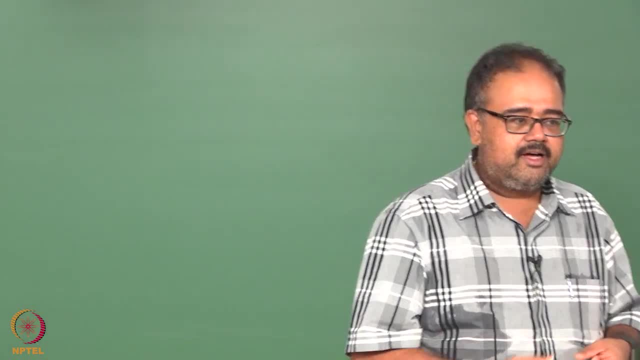 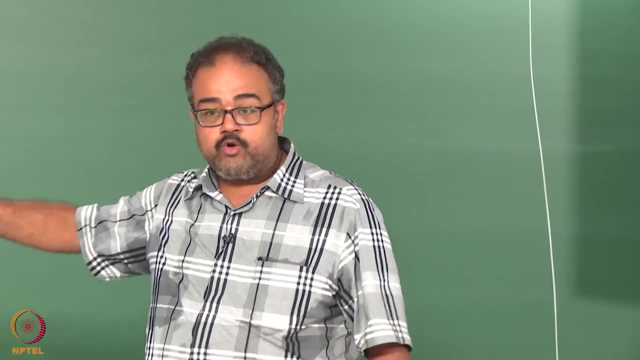 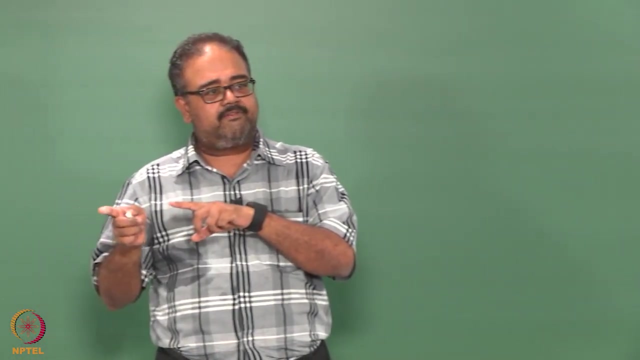 right. I am not trying to be too overly realistic here, but I am just giving you what are the factors that you have to take into account, right? So if you start talking about what could be optimal policies, right, then you are going down a dangerous path. that means you are going to start designing your problem itself, depending 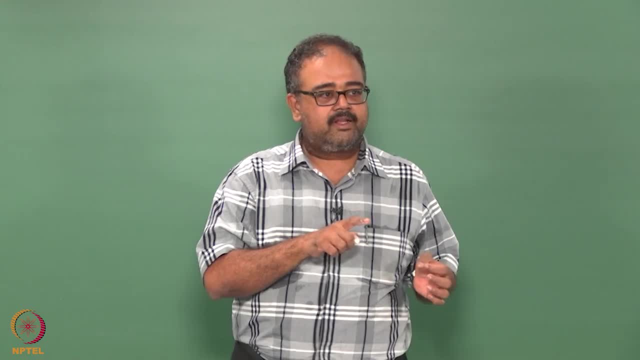 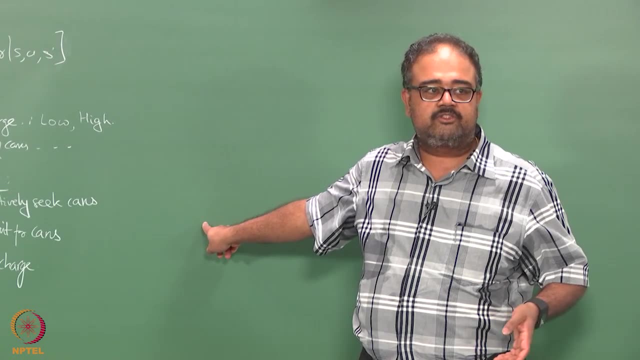 on what you think the solution should be, which is a bad thing. right, you should put in all the factors about the problem in the design and then you should go and let the algorithm figure out what the solution should be. So you should not start thinking about what the solution should be and then try to create. 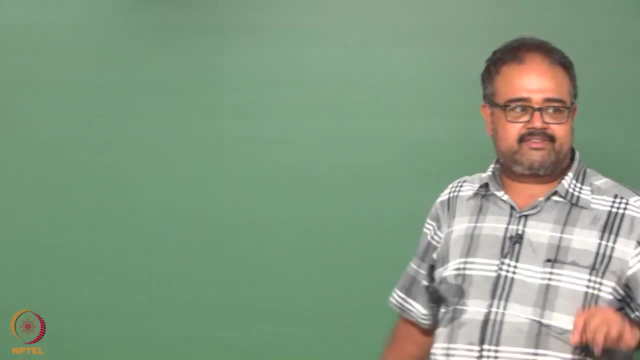 the rewards and the model itself. I will give you some time, Thank you. I will give you an example of that after I finish this. I will give you an example of when that became a problem. okay, So is it clear. 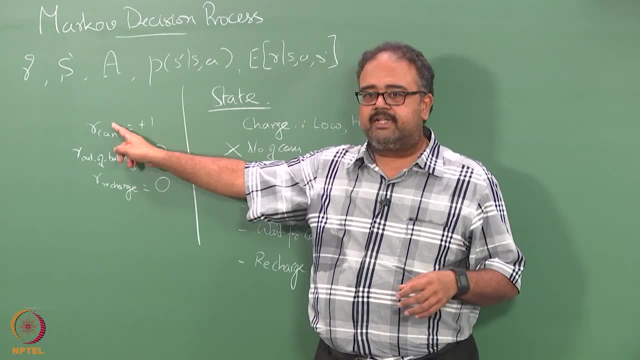 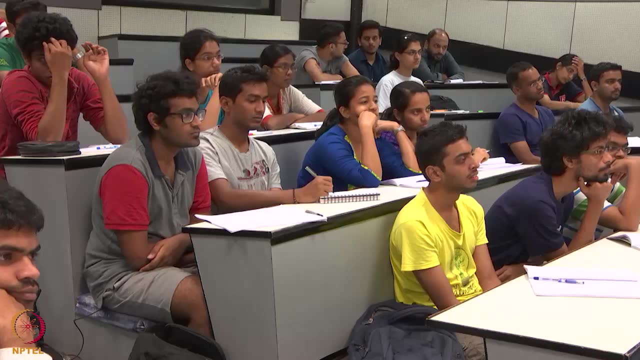 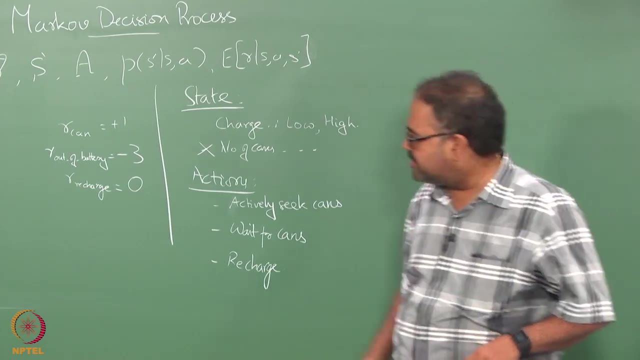 So now I need to figure out: if I actively seek cans, okay, what is the probability that I will get cans right? Is there anything else I need to know? Yeah, we will come to that. yeah, it is related to that. if I am actively seeking cans, what? 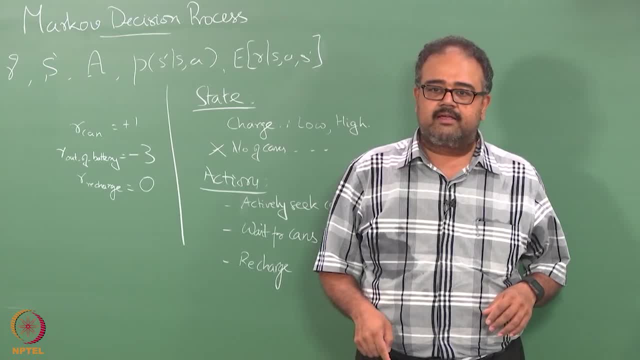 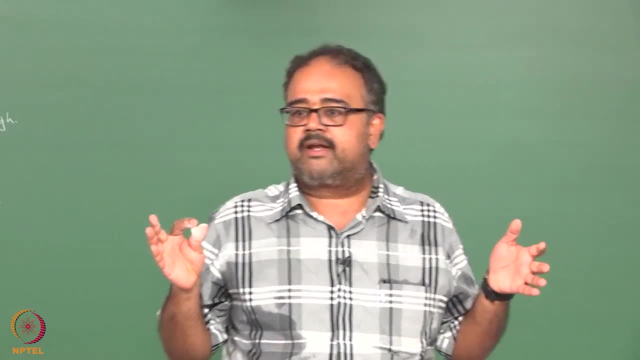 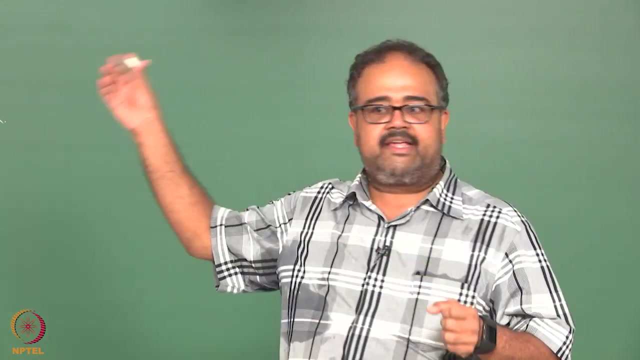 is the probability that I will run out of battery, because that also determines my reward, right? Or if I am waiting for cans to come, what is the probability I will run out of battery? maybe 0, because I have turned off everything and just waiting for, or maybe there is a leakage. 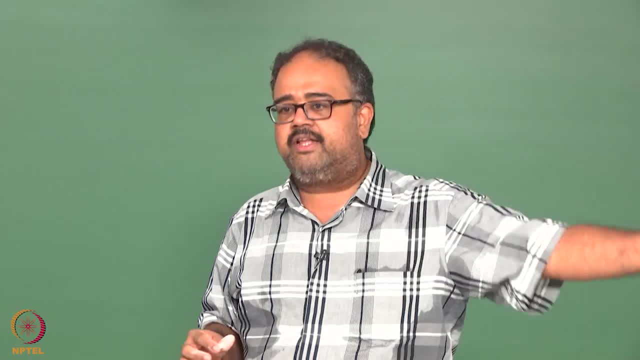 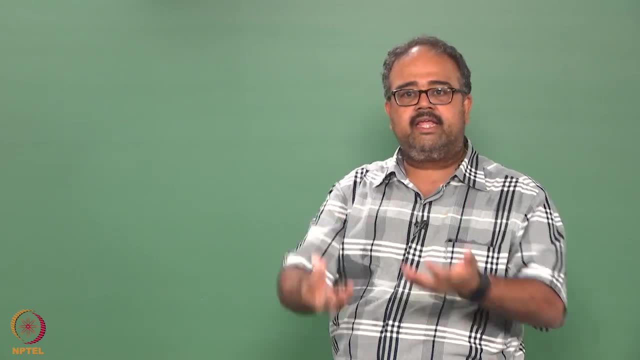 that is happening. Yeah, it is a very small probability that I might actually run out of battery, right. So I need both of these to actually figure out what will be the expected reward, right for a state action pair. so I need to know what will be the expected reward. 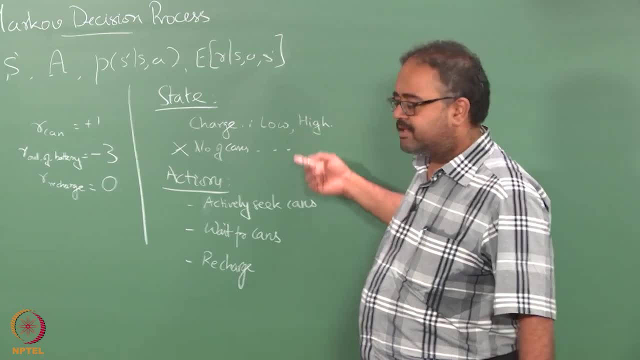 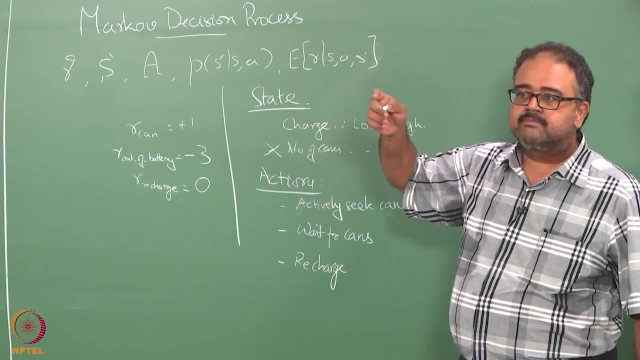 So I have to actually think about both of these. If I am in a high state, let at, I am actively seeking cans, right? So what is the probability I will find a can? Does it depend on whether I am in a high state or not? 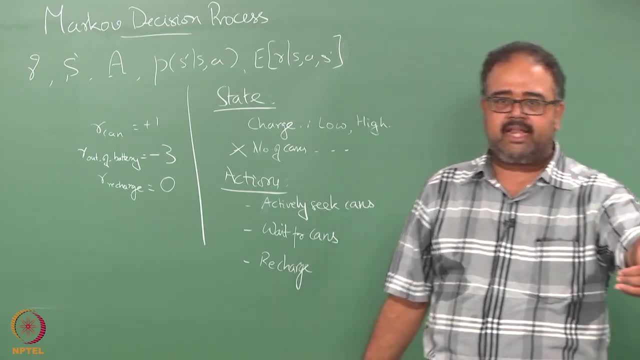 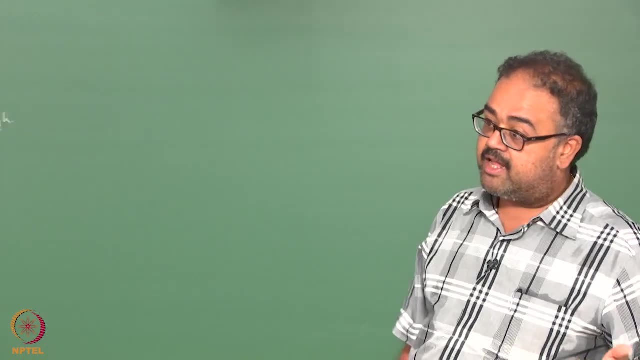 No, right. so if I am actively seeking cans, what is the probability I will get a can? okay, so that is one thing I need. Likewise, if I am not actively seeking cans, what is the probability I will get a can? that is second thing you need. on the other hand, if I am in a high state and actively seeking, 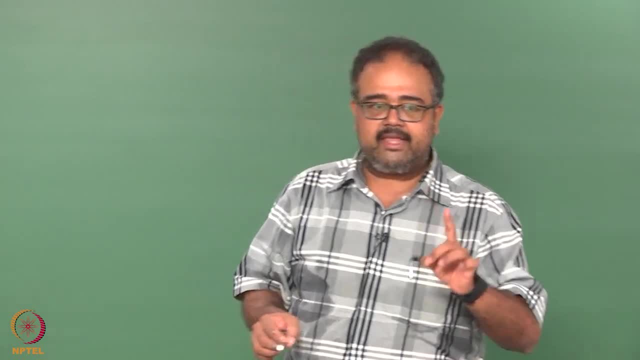 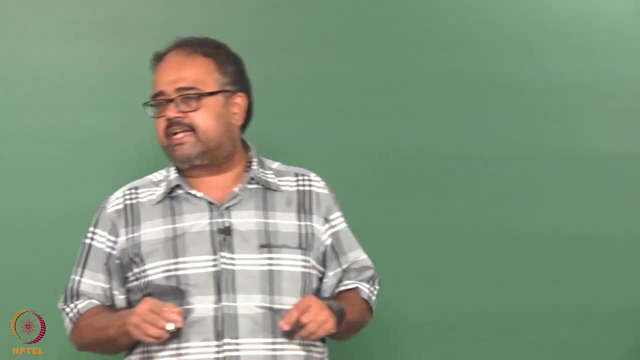 cans, what is the probability I will run out of battery? they are the state matters right. and likewise, if I am in a low state and actively seeking cans, what is the probability I will run out of battery? their state matters. likewise for waiting for cans if I am in a high state. 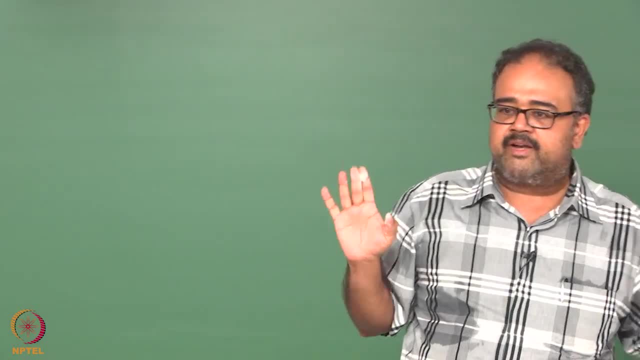 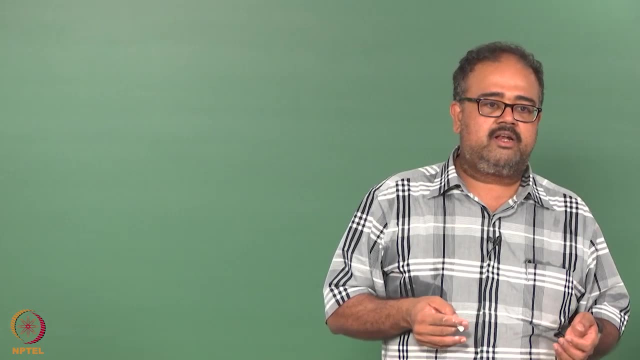 and I am waiting for a can. yeah, probability of me running out of battery is very, very miniscule, almost you know- but if I am in low state and I am waiting for a can, so even with the leakage power drawn, I might actually run out of battery. so these are the things. so 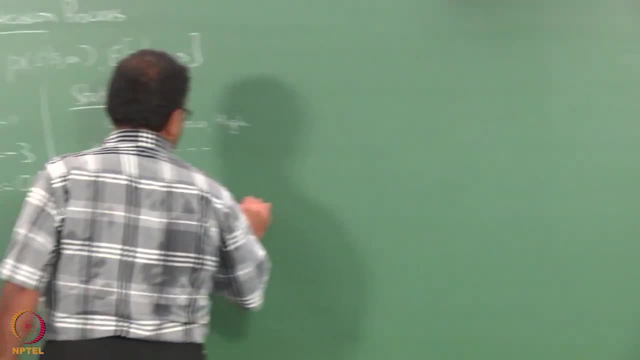 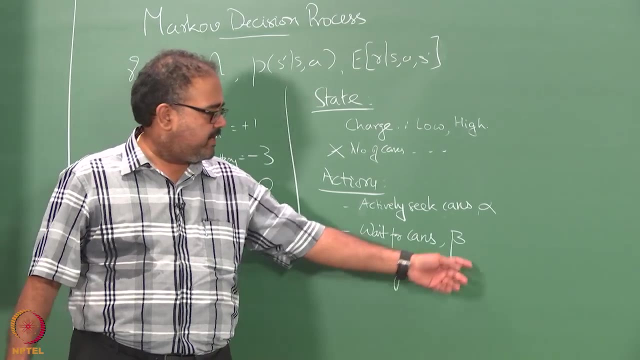 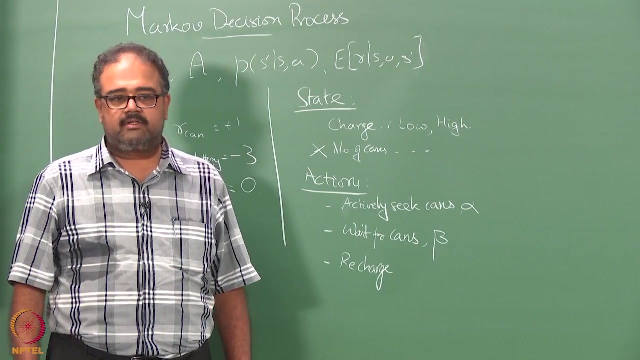 you need to know all of these right. for time being, I will say alpha as the right- the probability of you getting a can, right- and beta is the probability of you getting a can if you are waiting and then alpha is greater than beta. I mean hopefully typically right. this is talking. 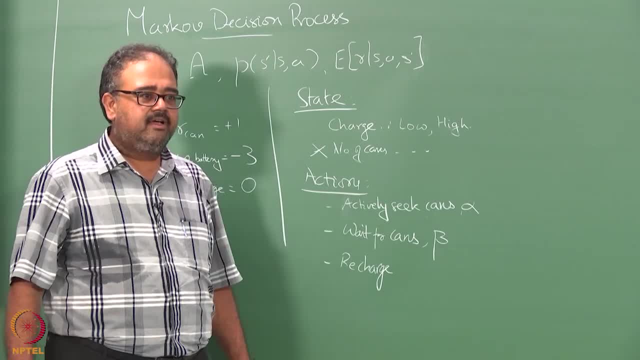 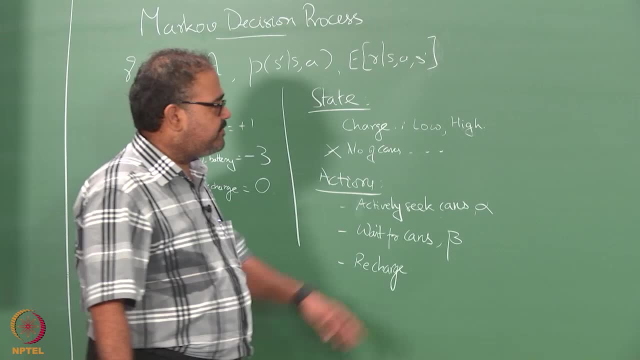 about probabilities. I mean that might be momentarily, I mean that beta is higher than alpha. like I said, stand outside a cafeteria during lunch time. but then overall, we are going to assume that alpha is greater than beta, since we have not actually modeled the time of day anywhere. right, we are just going to say alpha is greater. 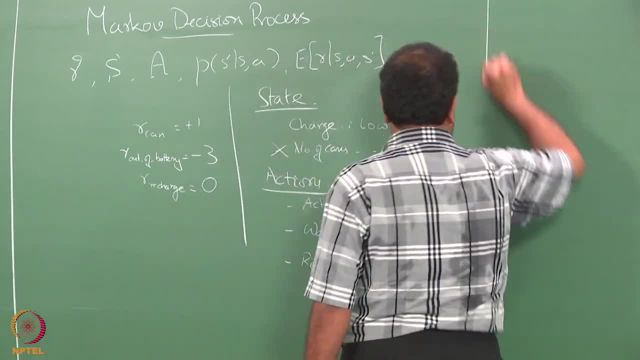 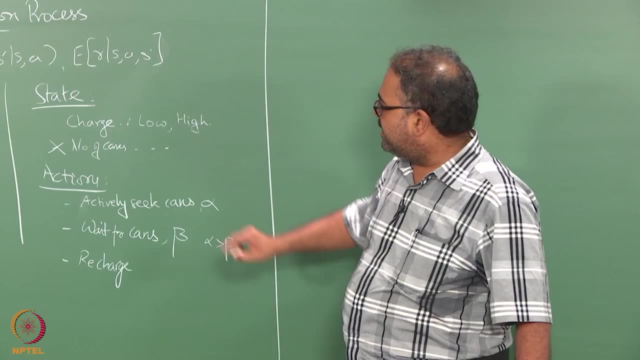 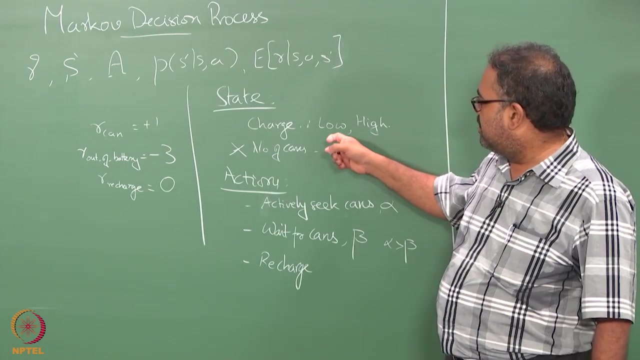 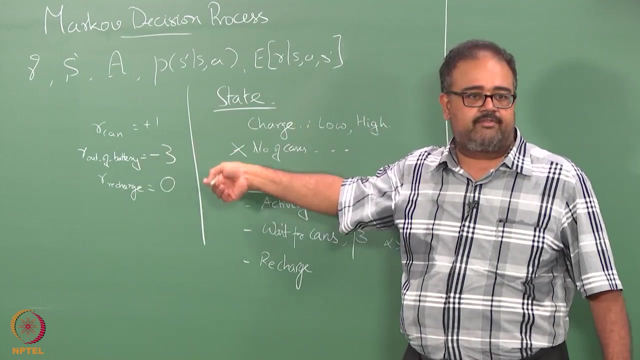 than beta, right? So now, what else do we need? yet we need to define P, right. So For that, what do we need? well, if I am in state high, what is the probability I will go to state low. okay, forget about going to out of battery. that is what we needed for the rewards. 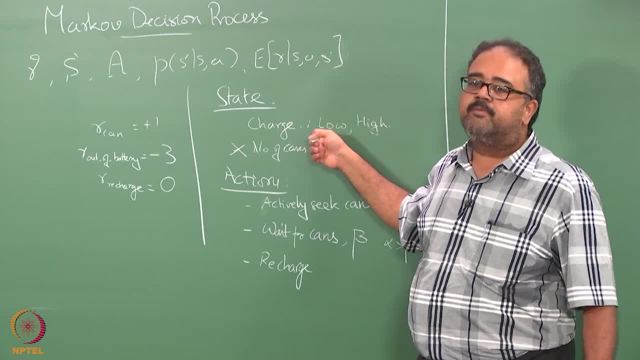 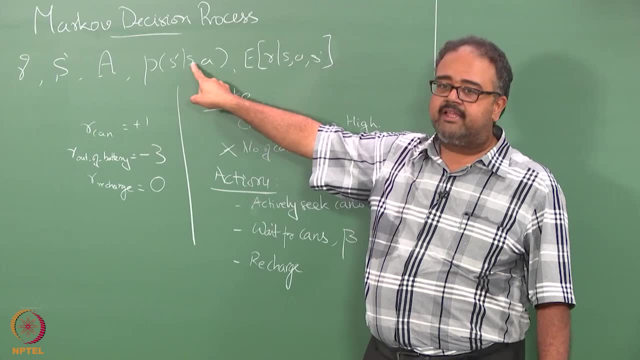 but for the state transition. so from high to low. what is the probability that will happen if I am actively seeking a can? so that is basically what we need, right? so I am in state high, I am actively seeking a can. what is the probability I will stay in state high? what 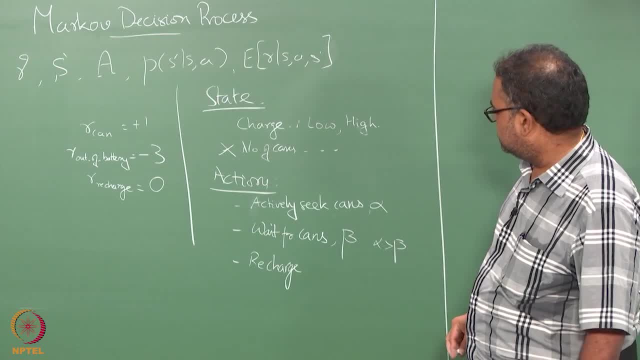 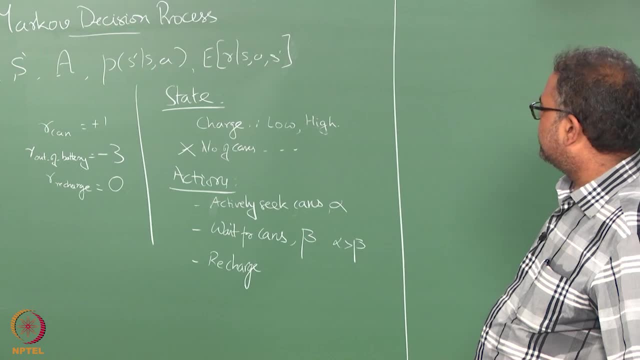 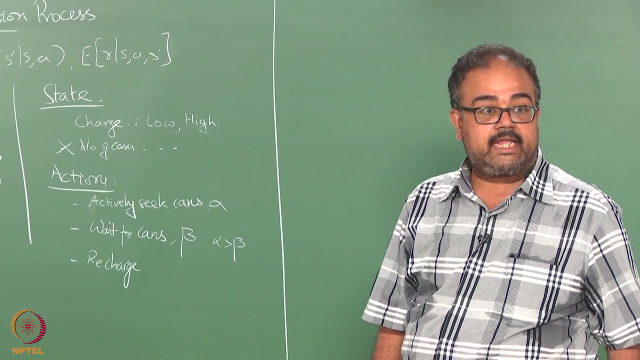 is the probability I will go to state low. right, Okay, Okay, Okay, Okay. So like that. and likewise, if I am in state low and I am actively seeking a can, what is the probability I will stay in state low? what is the probability I will go to state high? 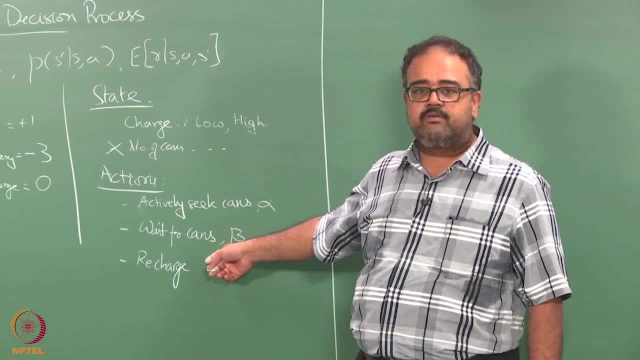 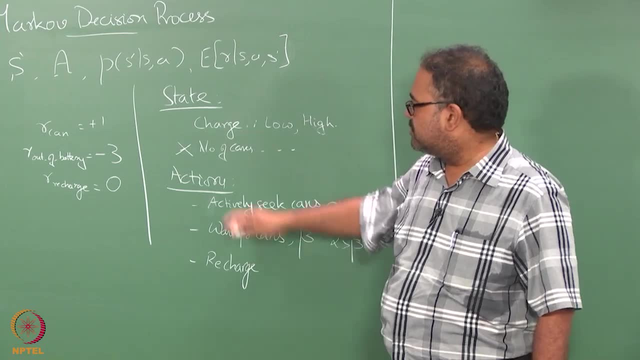 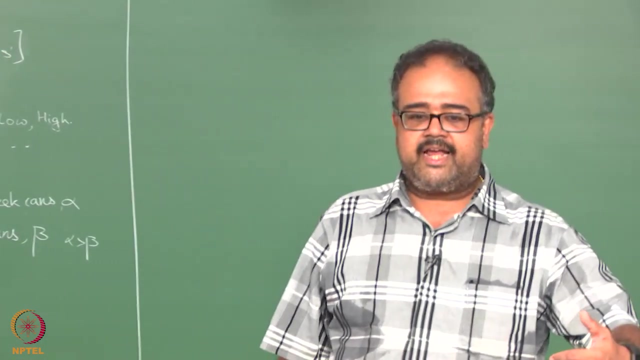 and I am in state low and I am waiting for can? what is the probability I will stay in state low? what is the probability I will go to state high, right and so on, so forth. right, So for defining the state transition probabilities. okay, of course, if I am in state high and I 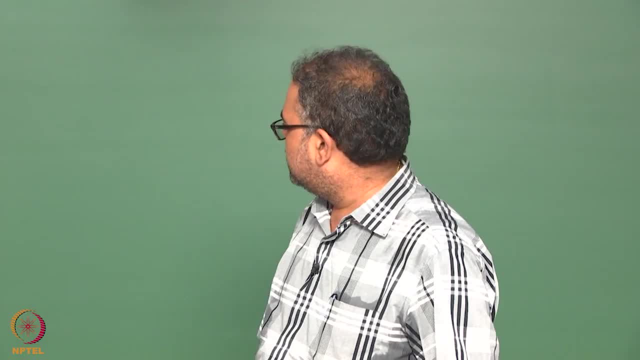 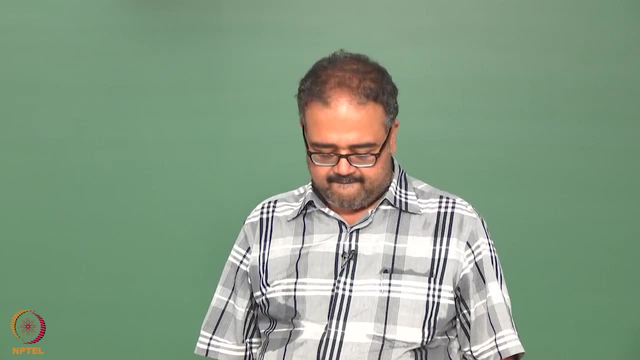 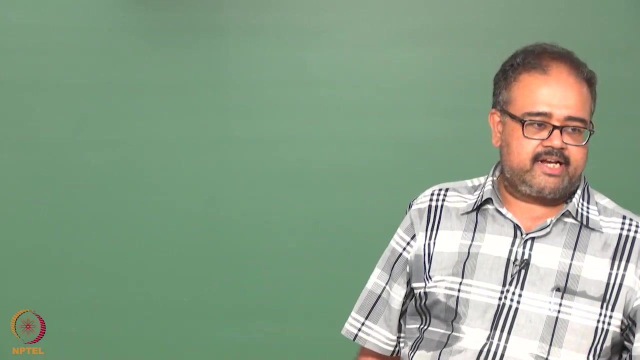 do action recharge. what do you want exactly? So if I am in state low, I do action recharge. with probability one I will go to state high, right, So we will actually prohibit recharge action in state high? well, it does not make sense. I have already fully charged, I do not want to go plugging in again, right? 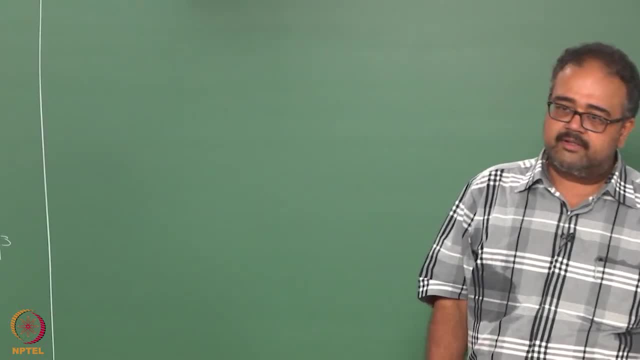 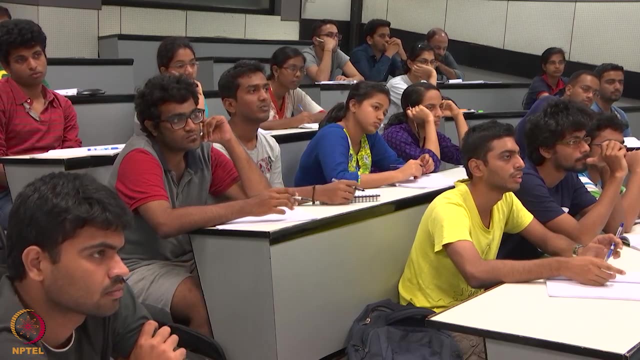 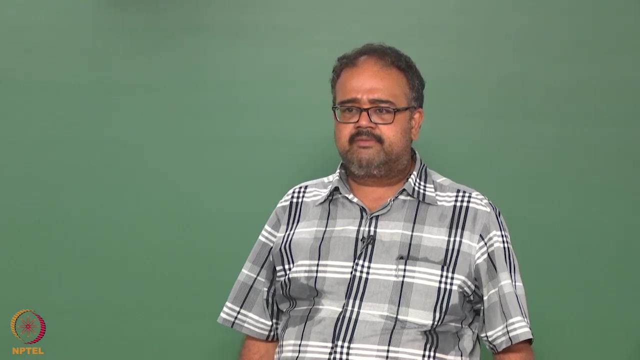 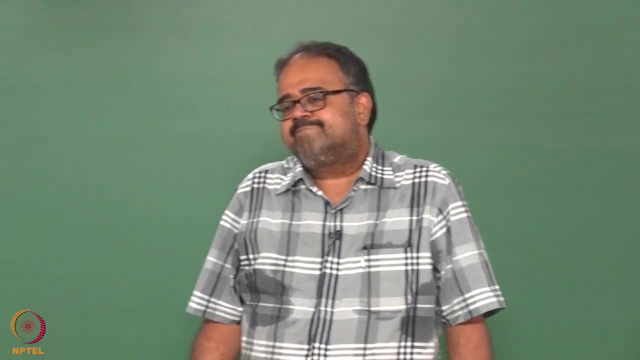 So I will, we will disallow that. yeah, well, all depends, right? I could just have a stochastic policy. I could say that, okay, my policy is that if I am in state high with probability 0.8, I will search with probability 0.2. I will just stay right. 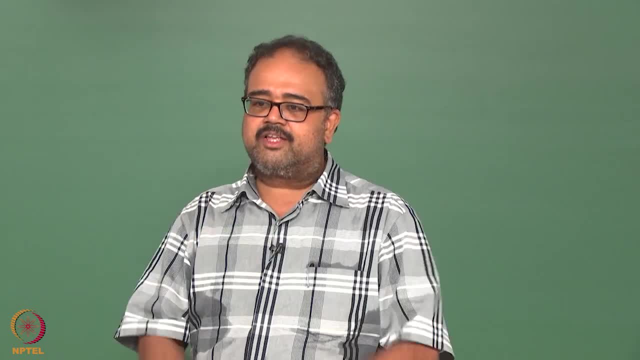 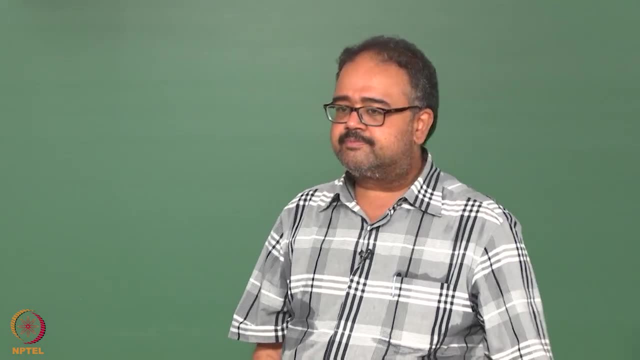 So I will do that. I mean so we are not talking about solutions here. I am just talking about defining the problem. this is what I was mentioning earlier. also, do not get into how the solution will look like, right? Sometimes you will have to think about how the solution will look like because you need 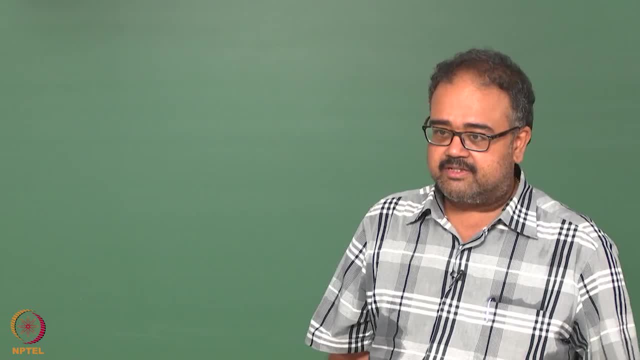 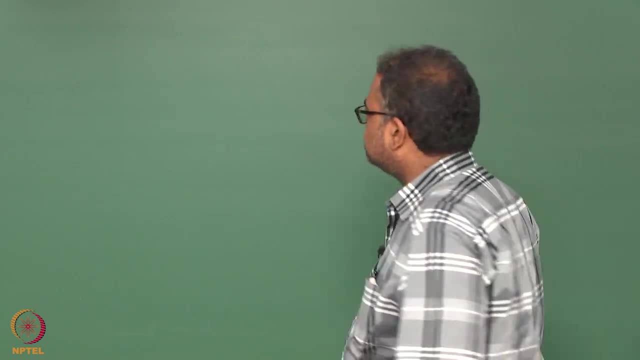 to know if you are giving the state sufficient expressiveness so that you know when the solution should change, and things like that. but do not worry too much about the structure of the solution. okay, So now we will just draw this, some kind of a state transition diagram. 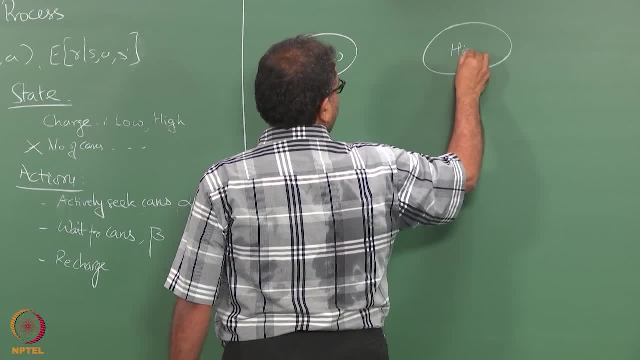 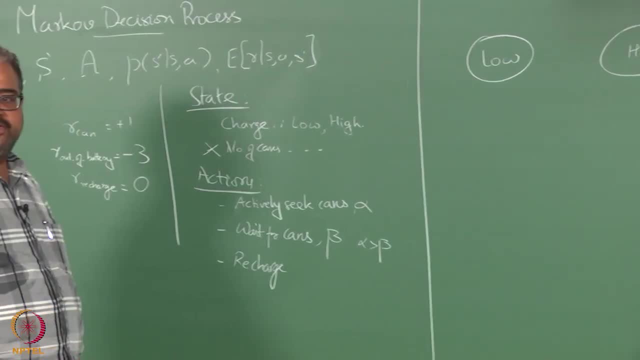 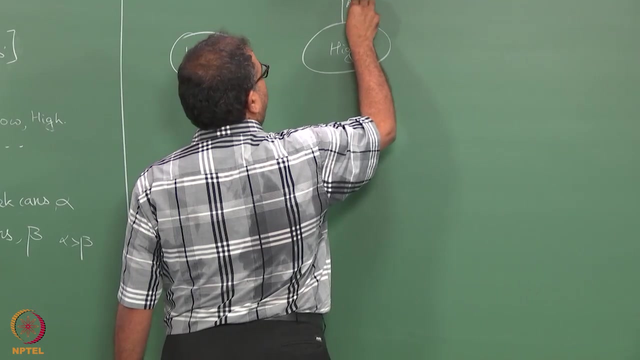 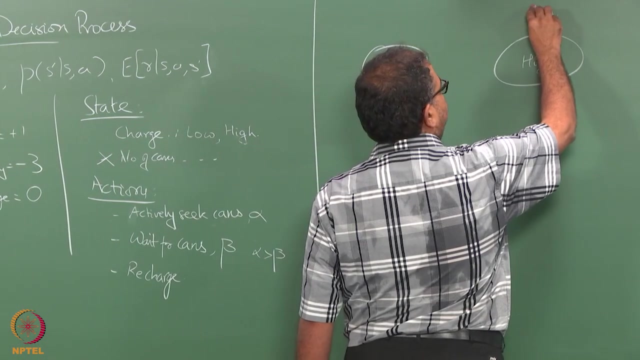 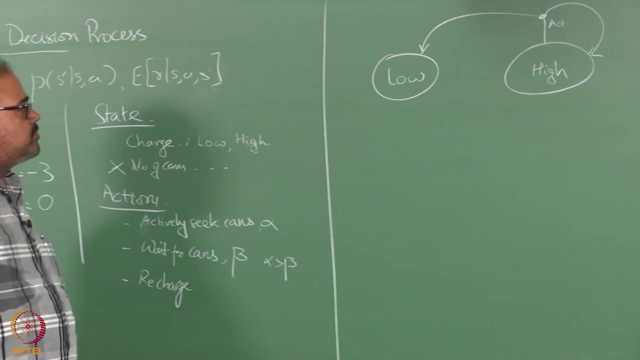 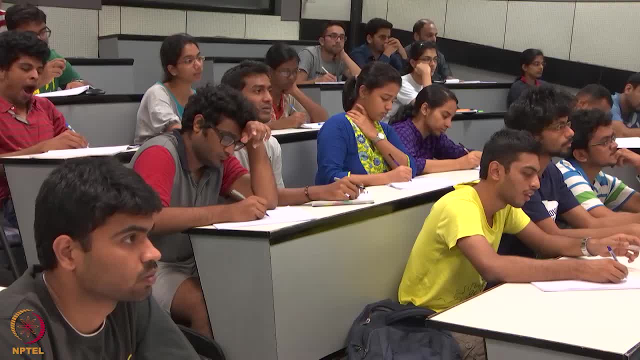 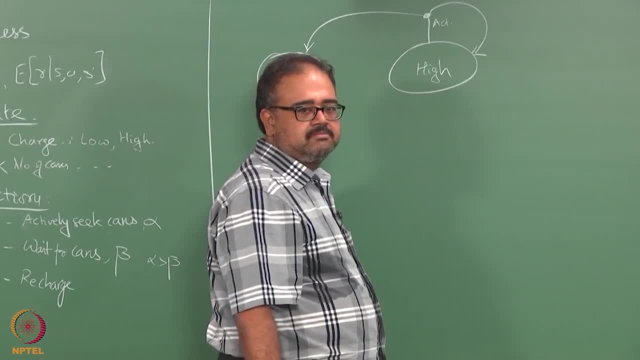 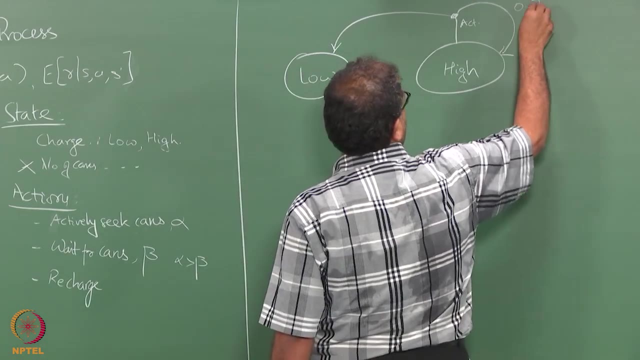 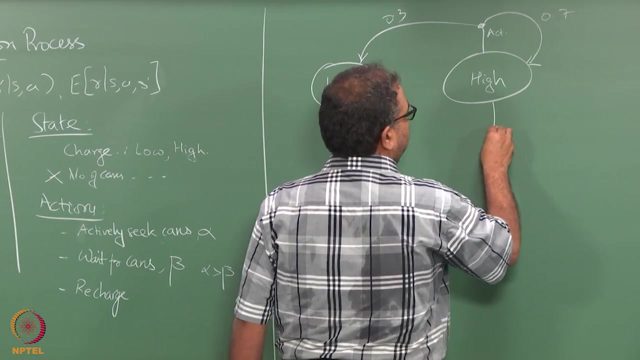 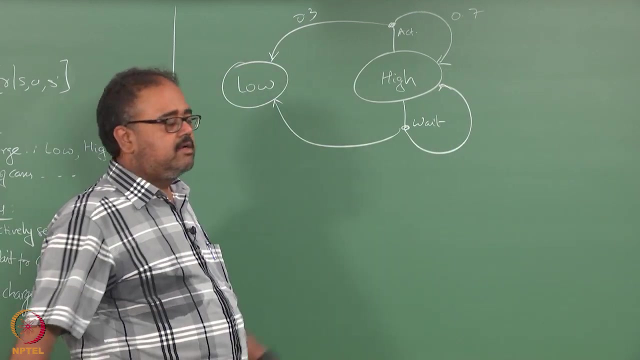 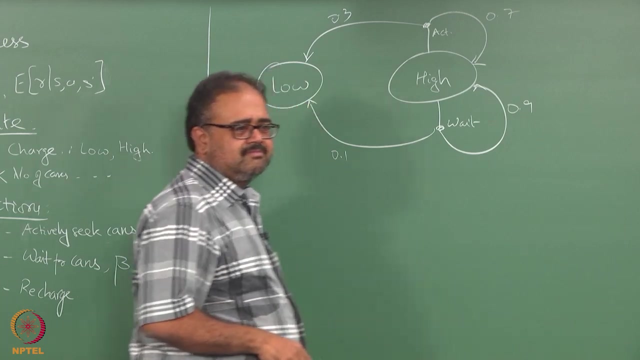 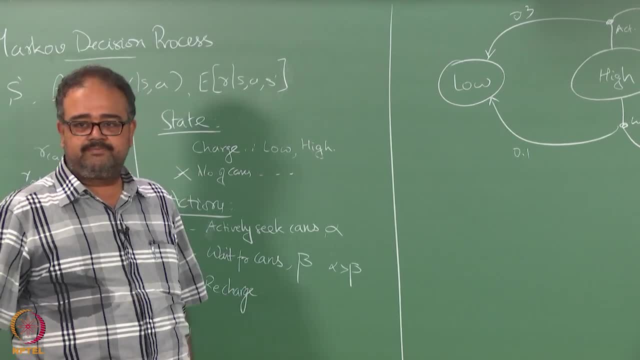 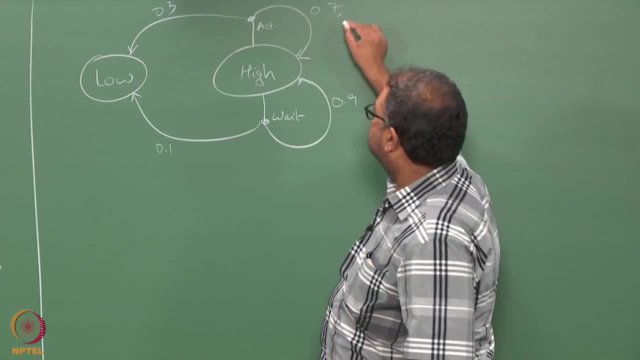 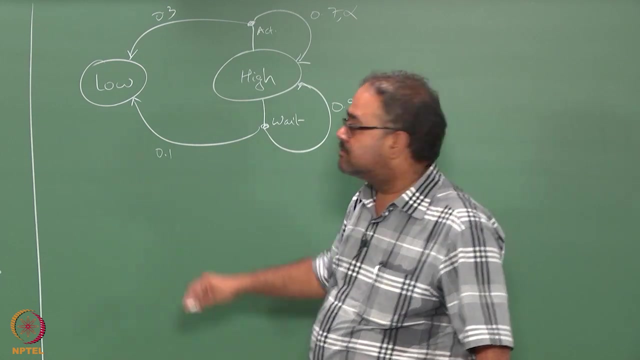 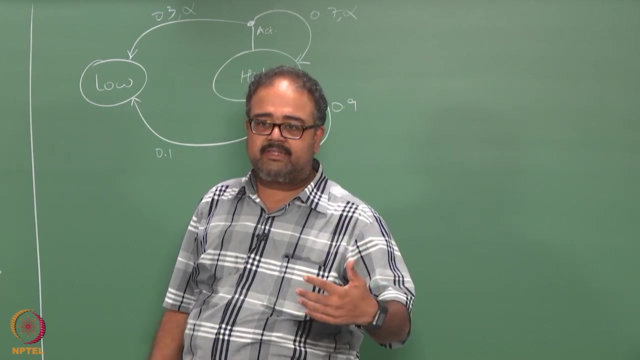 I need to look at what the reward is going to be for having done that right. So what will be the reward here? yeah, I will get plus 1 for a can, but the expected number of cans. I am going to collect this alpha right. there is a probability of me getting a can. 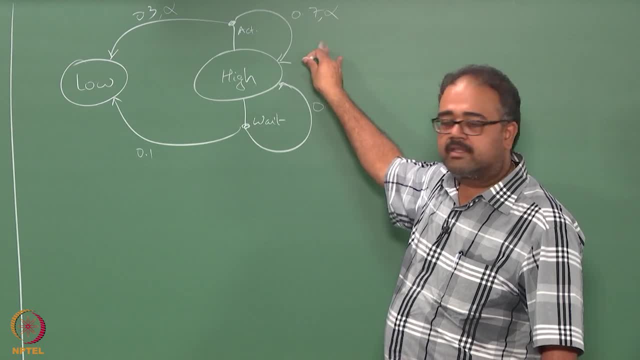 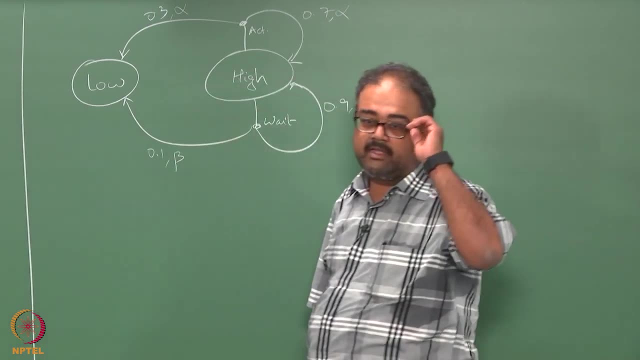 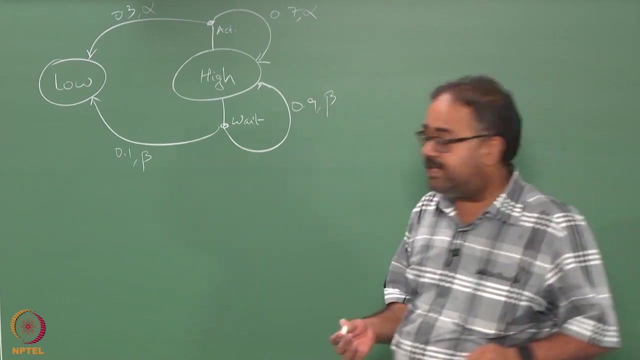 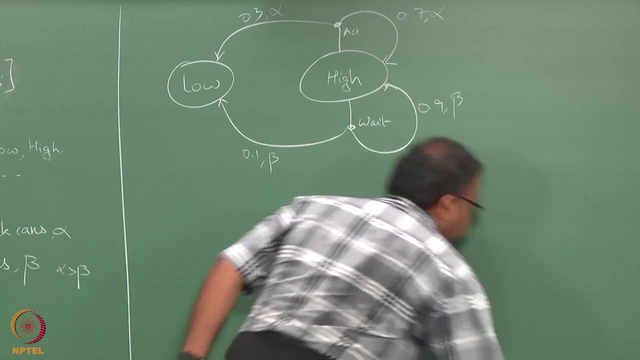 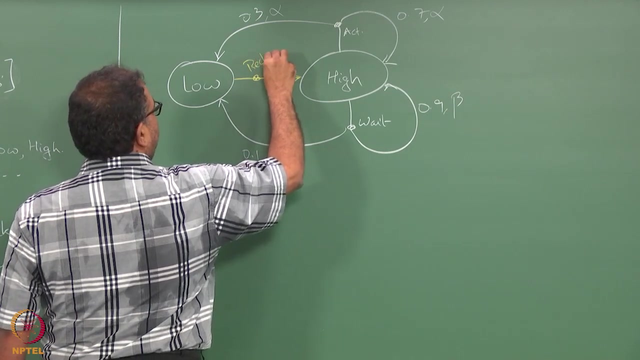 So the expected reward will be alpha right. likewise, here, the expected reward is going to be So: from low, I again 3 actions. from low, I have 3 actions, not 2. right, I have 3 actions. So what are the actions right? so I will do the easy one first. 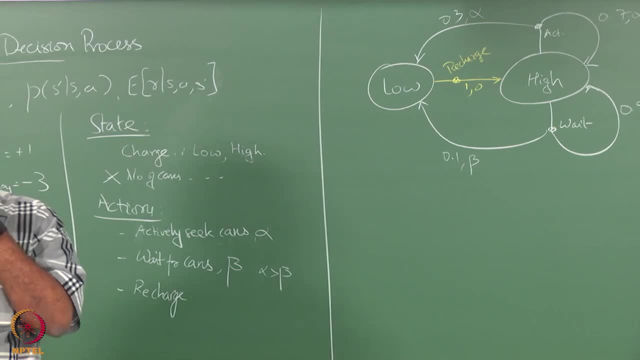 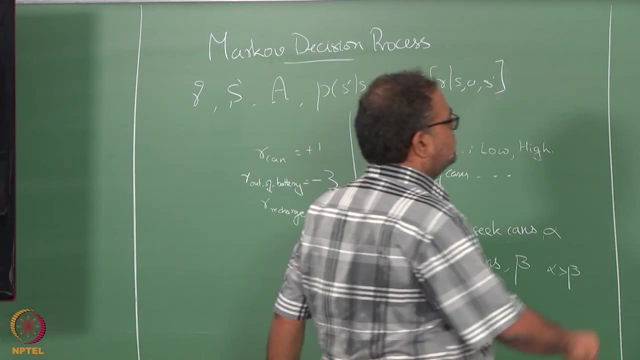 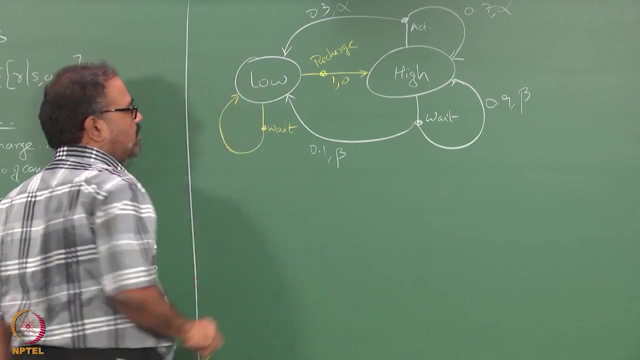 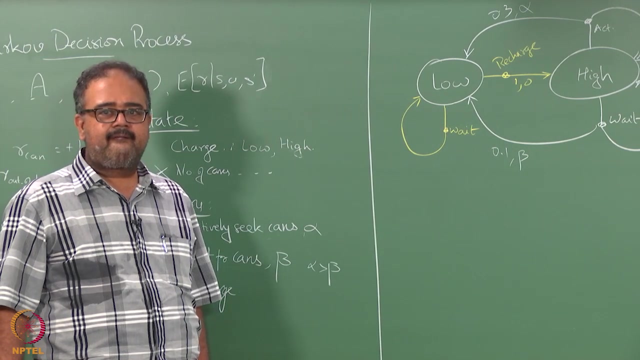 From low. if I do recharge with probability 1 I will go to high and I will get 0 reward right. so now comes the more interesting one. suppose I do wait here. is there any chance that I will go to high? I could right. 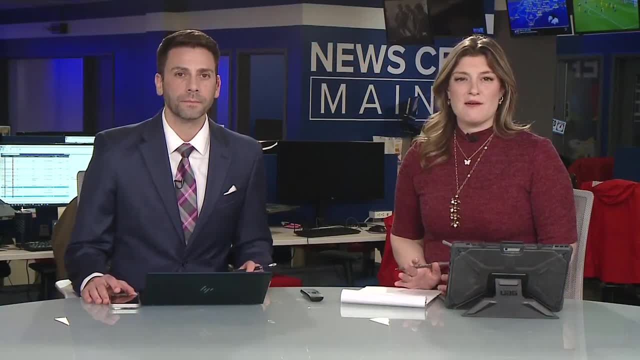 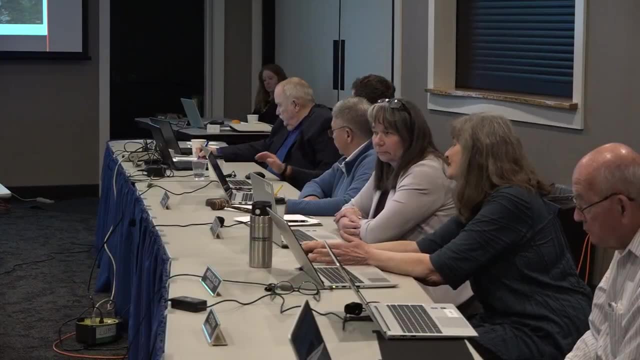 So today we're learning more about how some areas off Maine's coast could fare in a future impacted by climate change. Yeah, this morning staff at the Land Use Planning Commission presented a new report that forecasts the effect of sea level rise on certain island communities. On Matinicus Island, the assessment finds that two structures out of the 260 on the island could be affected if sea levels rise by around a foot, which the federal government predicts will happen by 2050.. On Monhegan Island, one structure would be affected in the same scenario. The authors of the report say the effort seeks to be the first step in understanding how to protect coastal Maine. 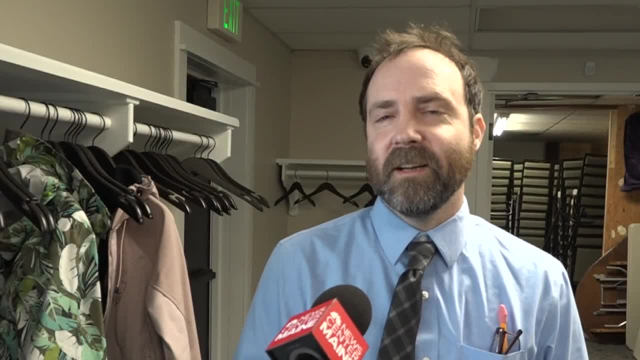 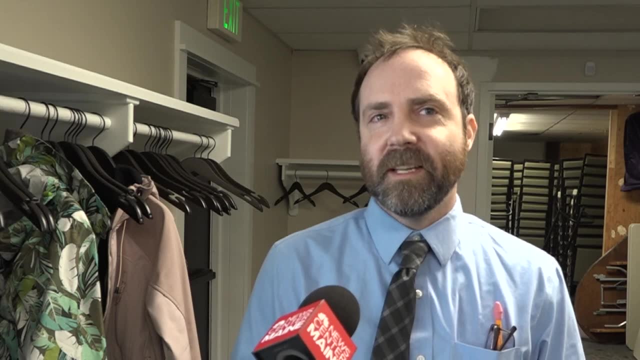 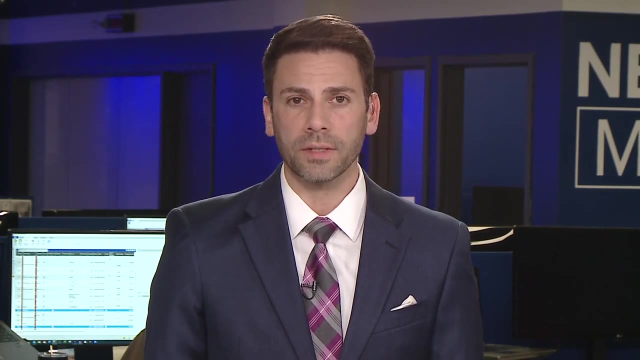 Folks are seeing the effects of these storms now, and the prediction is that, as sea level rise increases, the effects become worse, And so it's important to get a check on where we are now. The Land Use Planning Commission says the next step would be to visit the islands that the report focuses on, to then discuss mitigations.